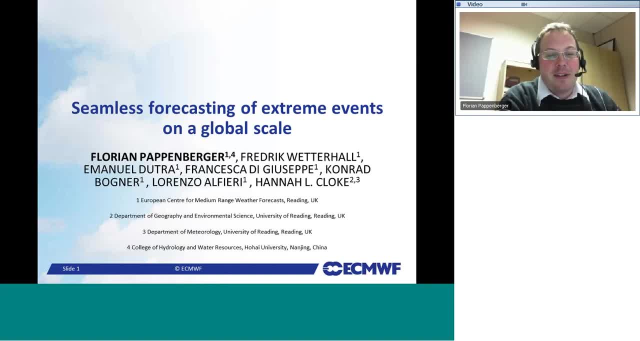 Seric puts everything up on YouTube afterwards, But given that we had already other speakers being put there, I don't think I can check them out. Seamless forecasting of extreme events. I think where I want to start is: just what do I mean by extreme? 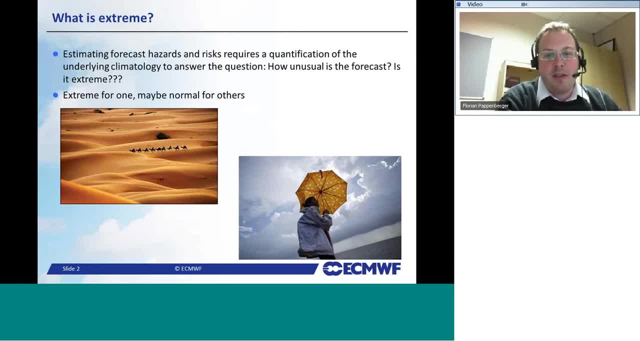 I think very often we talk about forecasting of extreme events And probably most of the time you've got some certain application or certain phenomena in mind. But realistically, I think we need to first think, or I need to first define what I mean. 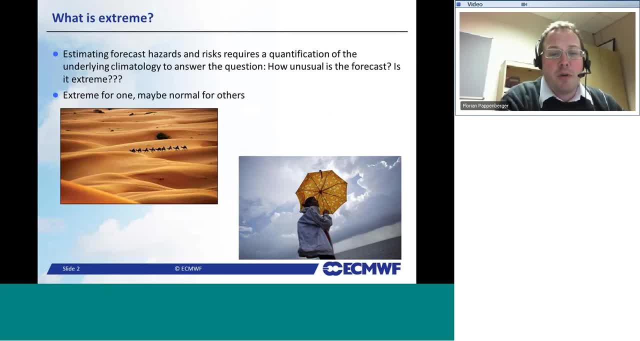 Particularly because extreme for one may be quite normal, And I've put you two pictures. I don't think that the people on this caravan will be too much bothered about the temperature, But if I would have that temperature now in Reading it would be fairly unusual for me. 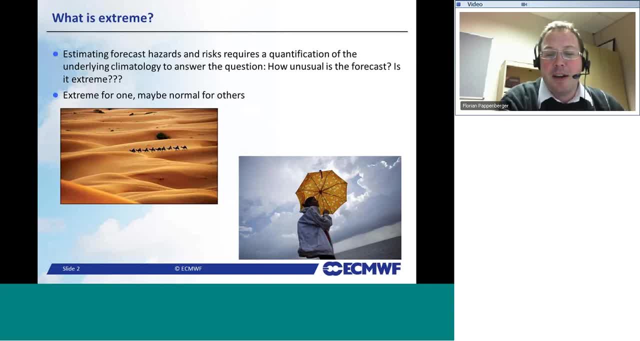 I can tell you I wouldn't be dressed for that one. Exactly the same, of course, for rain. For some people, having a rainy day and getting cycling home in the rain may be completely normal, Whereas for others it's probably an extreme. 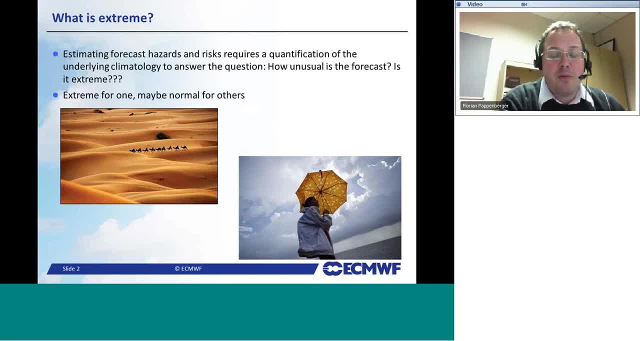 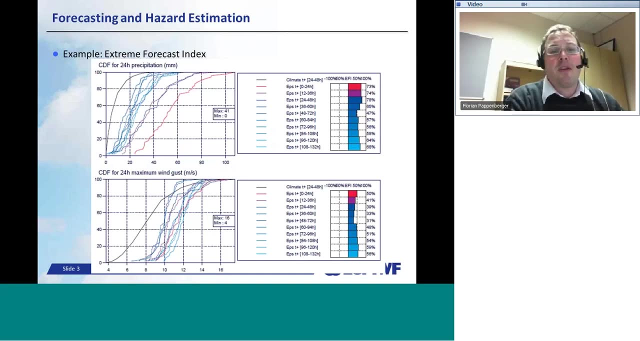 And, of course, you can spin this forward Further and further. Therefore, I do think that, in order to estimate extremes, you actually need to set this in context. You need to set this in context to an underlying climatology, To something you probably think would be more normal. 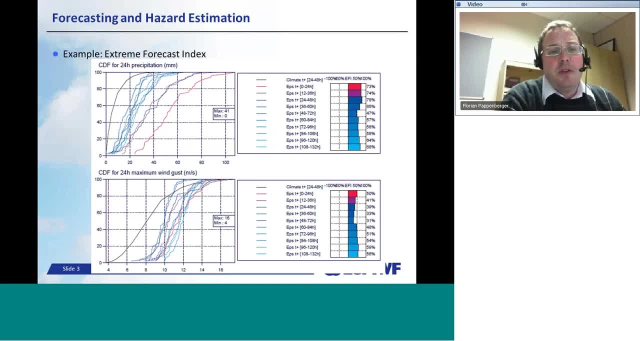 And here I've taken an example which we use in ESMWF, which is called the Extreme Forecast Index. The Extreme Forecast Index is designed to give you an indication on how extreme that weather is in relationship to climate. So what you see on this plot is a CDS. 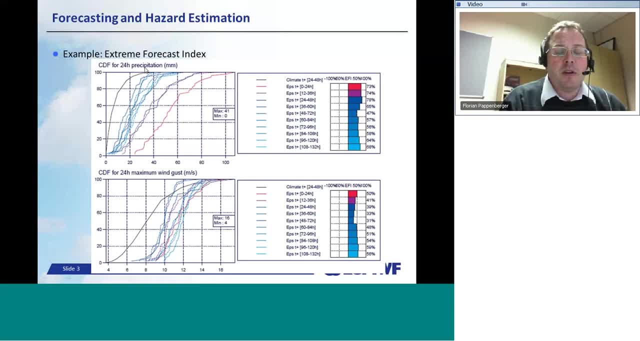 The black line is the climate distribution. By the way, this is actually a presentation forecast for the Philippines just before the disaster, And what you see here in red lines or in purple and blue lines is different lead time forecasts. It's a distribution of the ensemble. 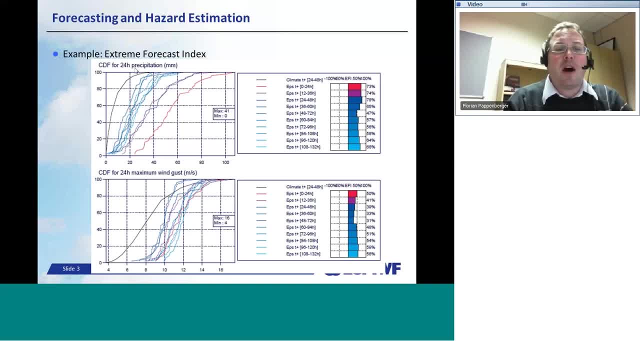 What we have here at the top, The top plot- is 24-hour precipitation accumulated. At the bottom we've got 24-hour maximum wind gusts And, of course, the more on the right-hand side your ensembles are, so the more away they are from the climate, the more extreme is it. 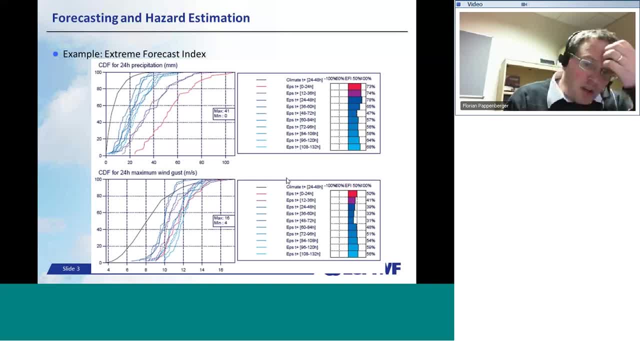 The same for the wind gusts, And you can see here for this particular example, in the beginning, maybe the lead time of four or five days- there was an extreme indicator for precipitation, And then you've got more and more extremes the closer it gets to the event. 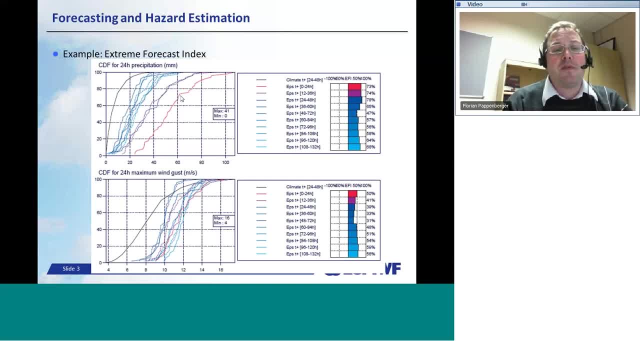 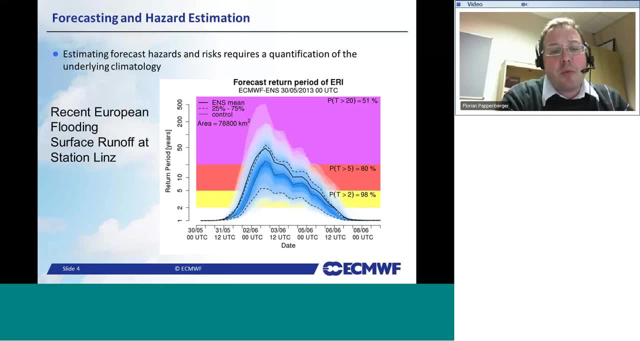 And at the red line. it's really completely different to what we would expect as a climate. This would be one way of defining it. The other way, where we probably often more think about, is in terms of return periods. Return periods are also related to an underlying climate. 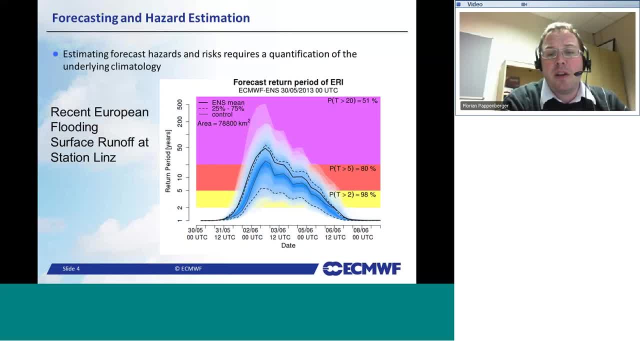 And here's a plot from the Extreme Runoff Index from Lorenzo Alfieri For the recent European flooding: surface runoff at a station limped And you've got nicely here in the y-axis a return period starting at one year, going up to 500.. 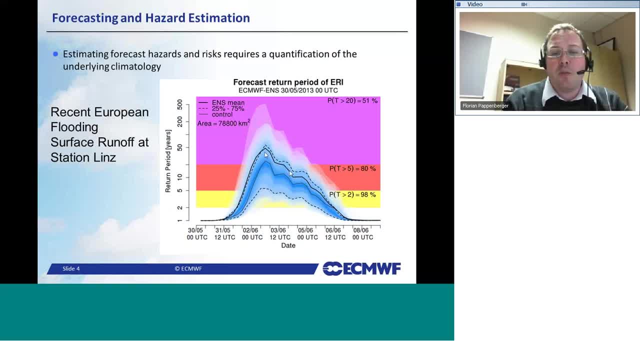 You've got a forecast of ensembles And you've got three different warning levels in the upstream area And that would also be a way of trying to give you a feeling of how extreme that discharge is. If you look at that particular discharge, you can see that actually, in comparison to this return period or this climatology, 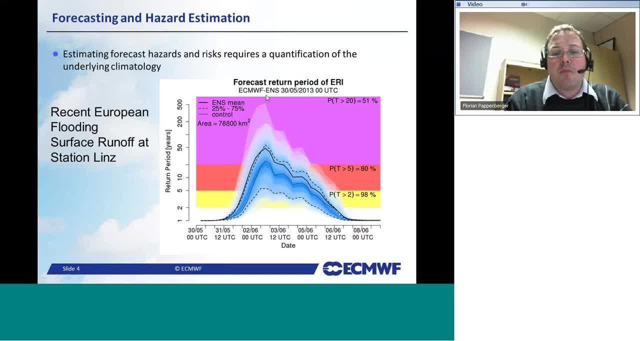 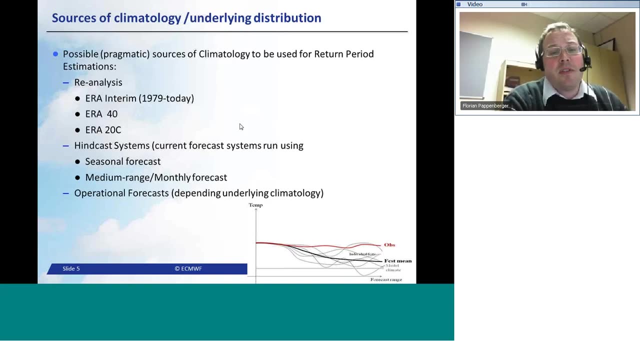 there has been quite an extreme predictability of this, Or there has been a large number of ensemble members indicating a return period of more than 20 years. Having said that, climatology always sounds like a very nice concept, People say, oh, we compare it to climatology or the underlying climatology. 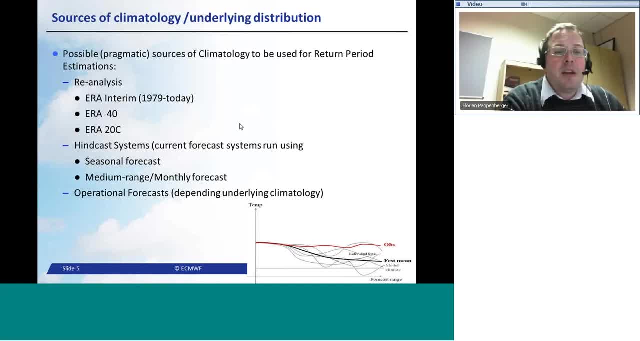 However, there's many pragmatic solutions, or there's many solutions for climatology- And I'm deliberately not showing you any station data Or direct measurements Because I'm trying to talk about a global, more large scale type of approach And pragmatic solutions. here I've listed three. 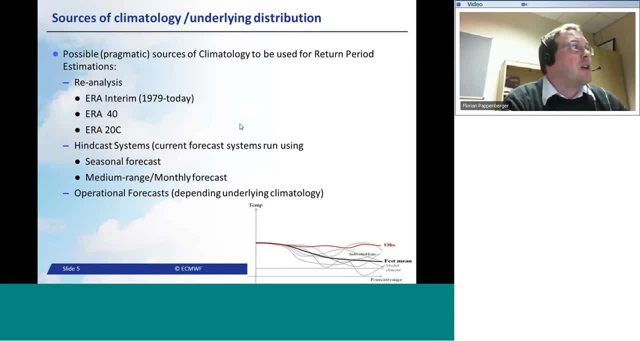 It could be the reanalysis. So the reanalysis which gives an indication of how the climate is Era interim, Era 40. Or the new one which is called Era 20c. It could be hindcast systems, which is the current forecasting systems that have been run for a certain amount of time. 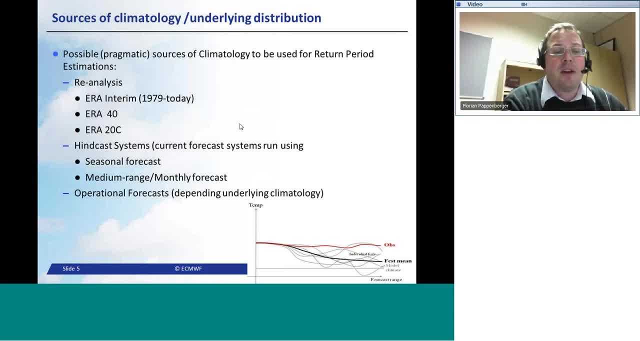 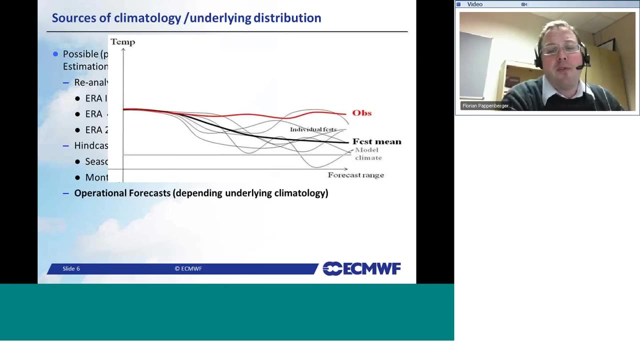 For a certain number of years, for past events. We have that for the seasonal forecast and the medium-range forecast, Or it could be also the current operational forecast. We've got a forecast. different ensemble members. Here's the observation, Here's the model climate. 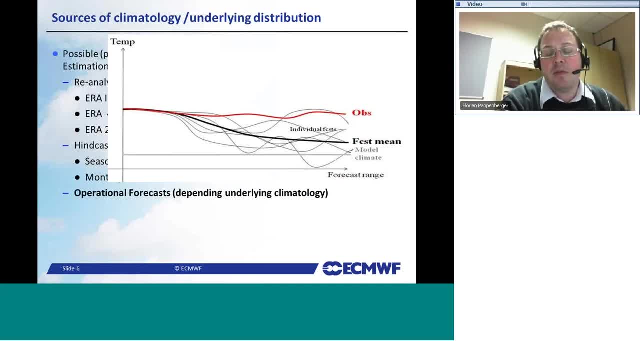 Any forecast at some lead time drifts back to the model climate And you can see it quite nicely. Of course, you can use this effect in order to build up your climatology. This is a distinct advantage over the two previous approaches. The hindcast systems are very often smaller. 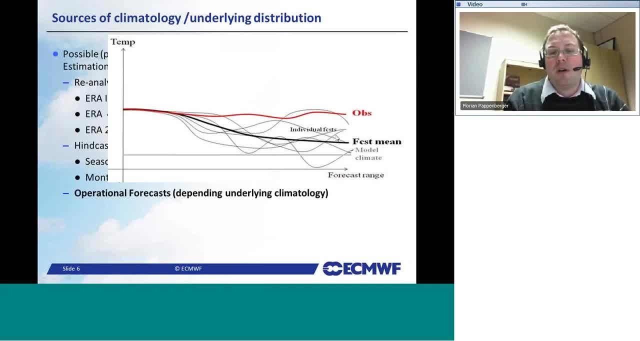 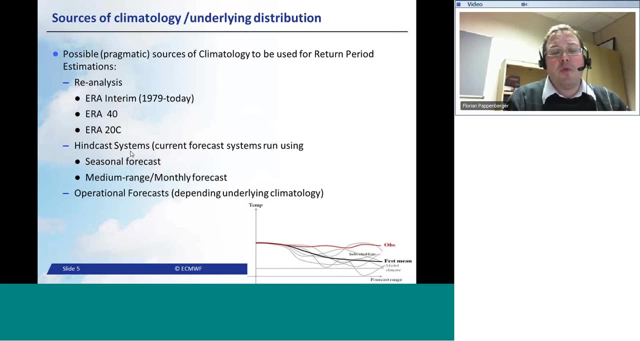 They're very often restricted to how much somebody can run on their big computers. The reanalyses are very often very sets, sets, sets. Era interim goes from 1979 to today. Era 40 goes on to 2001.. And Era 20c starts at 1900 and goes on to today. 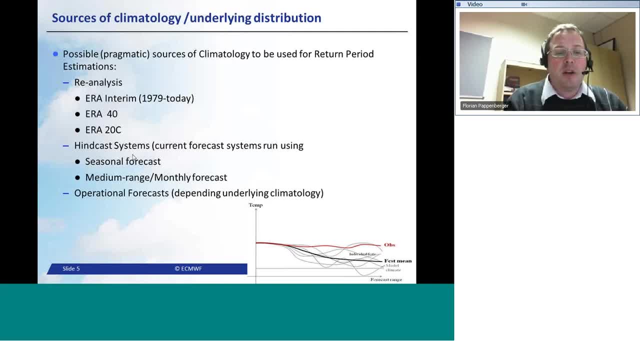 But they all have a very distinct advantage: They have a very limited set of samples And very often they're based on an older model, An older model, climate, An older science. Because they're so expensive to do, The operational forecast has the advantage. 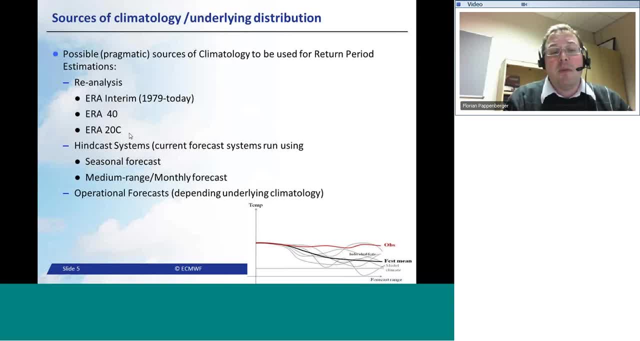 It's produced every single day, So usually you tend to have a larger sample, Although you don't have a larger sample in time. I'm not just talking here theoretically, I'm just listing here a few examples where these climatologies have been used. 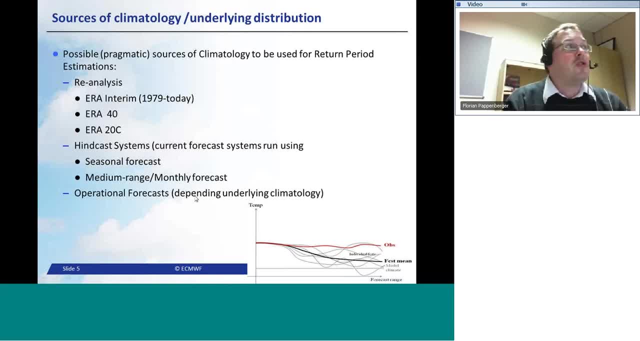 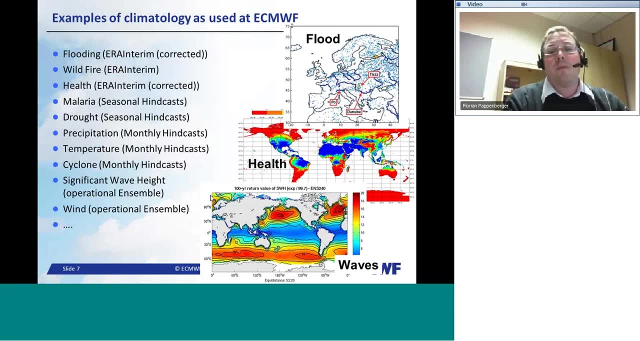 In WF We've used or we've built up climatologies for flooding, wildfire, health indices using era interim And you've got a nice plot here of, for example, flood inundation map based on corrected era interim. Similar here is a health index. 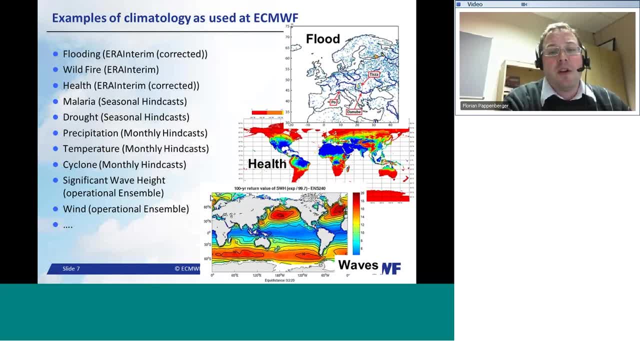 So up here in the flooding you see flood and extent. In the health index you see severity of flooding. But it's based on era interim. You could use the seasonal hindcast system. We start this with malaria and droughts- The monthly hindcast system. 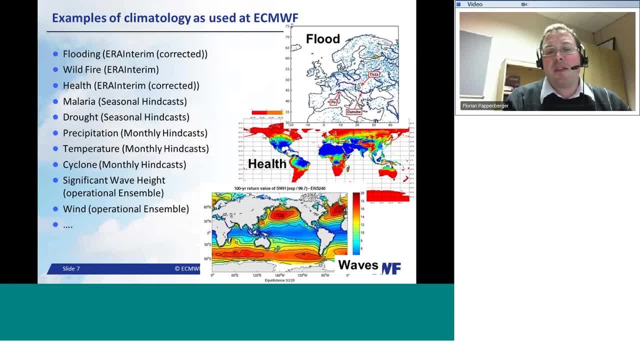 Presentation temperature, And you've already seen an example of that, because the extreme forecast index is based on that. And then, last but not least, we have this concept of using operational samples, And we've done this in significant wave heights, And what you see here, for example, is the 100 year return period of a significant wave. 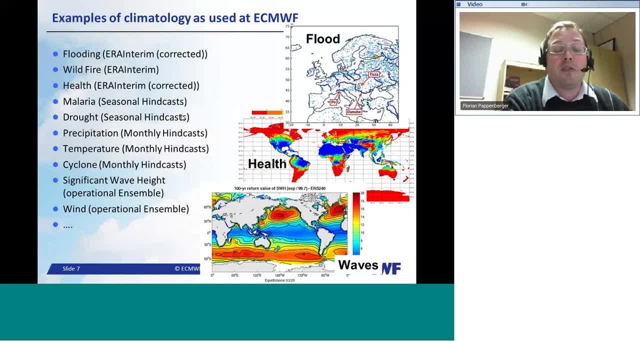 height across the oceans using that concept. Having talked a lot now about how to build up an extreme forecast, I want to get to. what kind of extremes do I want to talk about today? We've done quite extensive tests here and tried to figure out where is our forecast. 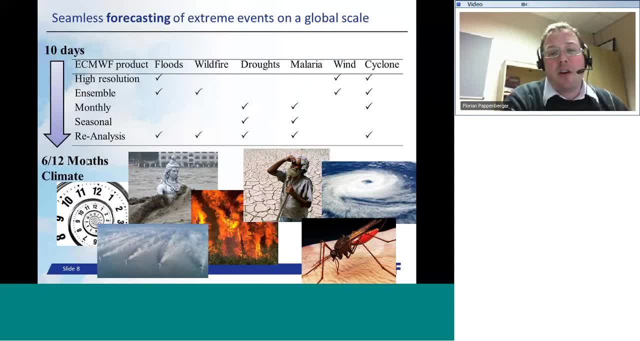 valid and useful in terms of forecasting, And I've mentioned only six different areas now- Floods, wildfire, droughts, malaria, wind and cyclones- And we use different types of product depending on the type of phenomena. For the more short term, we use the high resolution ensembles forecast that normally goes up to 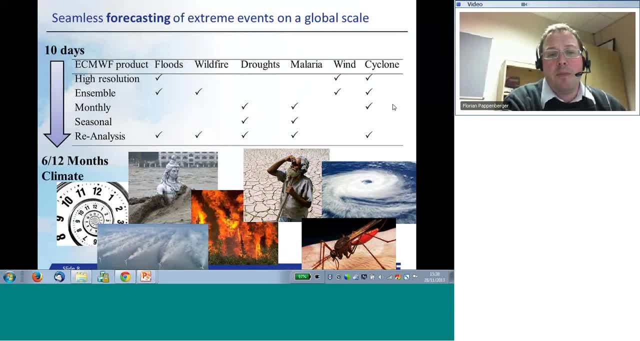 ten days. For the more longer term, we use the monthly seasonals between 30 days and seven months forecasts, And then very often we also use reanalysis to create additional conditions. I was a bit too ambitious when I wanted to do this talk together. 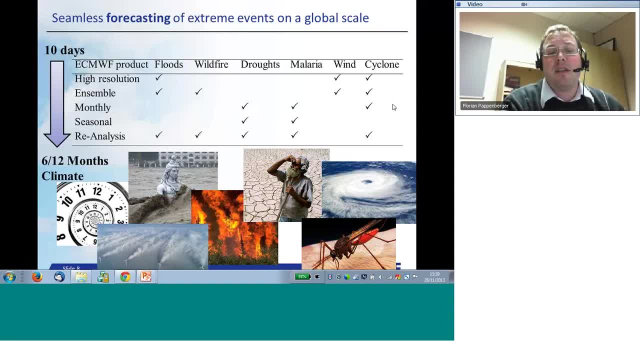 And, as I said, I'm not a scientist. I'm not a scientist, I'm not a scientist. And when I put it together I realized I've got a bit too many slides. Not that unusual for me, But therefore I'm only going to show you some examples now of floods and droughts today. 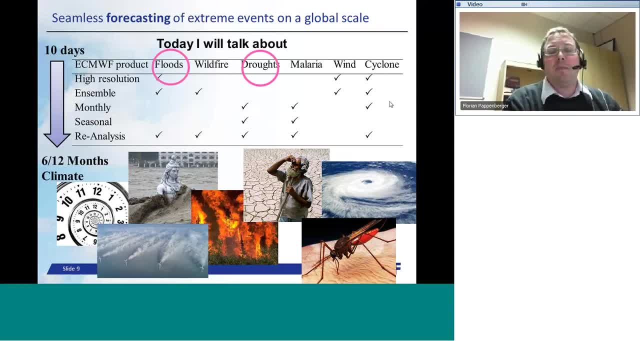 If you want to have the rest, either, get out your mobile phone now. At the bottom you see this QR code. You can scan it in. It will be in a few slides from now on coming, so you have enough time to do it. 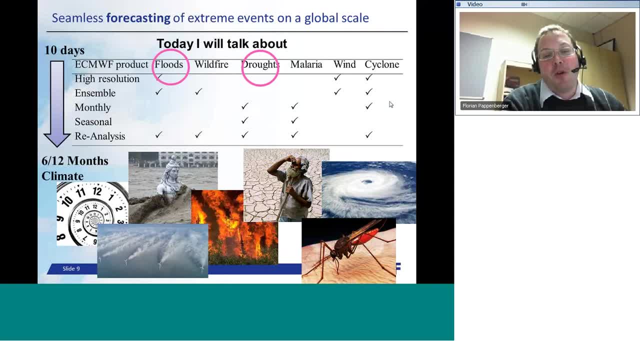 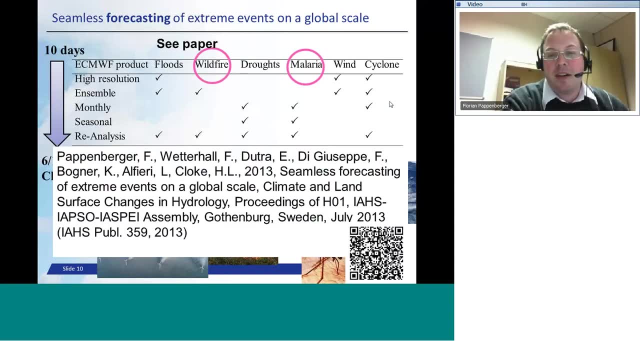 Or you just search for this paper, which is listed here: Wind and cyclones. I'm not having a dedicated publication. It's part of the ETHNWF normal product and I think I'd be able to point you to the right publication. Just drop me an email. 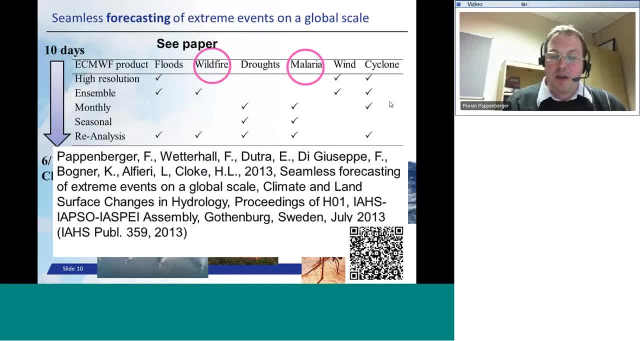 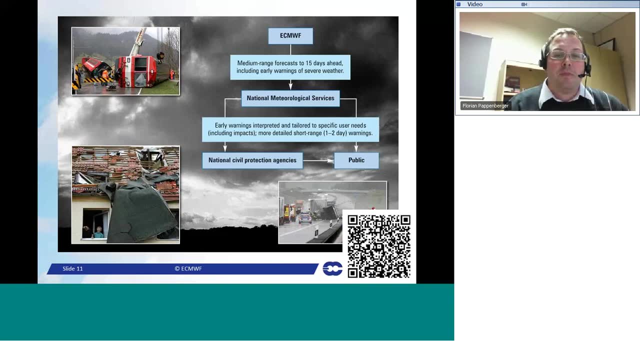 The question is always why we're doing this. ETHNWF is a medium-range weather forecasting service and not an extreme warning or not a warning agency. However, our remit is including early warnings of severe weather in support of the National Weather Service. 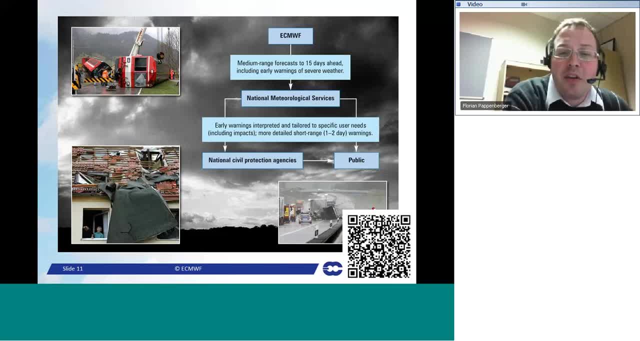 So what I want to do? I want to demonstrate the value we have using ETHNWF forecasts for these types of severe weather, and then it's up to the National Weather Service, the National Civil Protection Agencies and public to go from there. I think. in order to give you some setting, I decided to start and just talk a bit about. 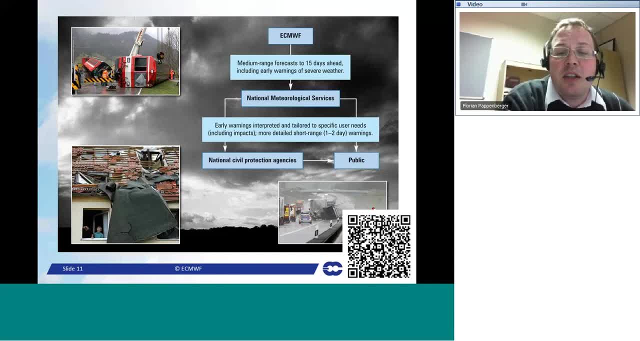 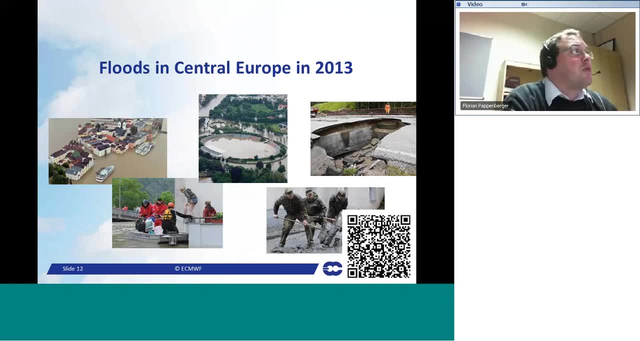 the floods in central Europe in 2013.. Okay, So I'm going to start with the flood forecast. Some of you may remember there's many reasons. All my examples are based on the European Flood Awareness System. This is a system which produces medium-range flood forecasts across the European continent. 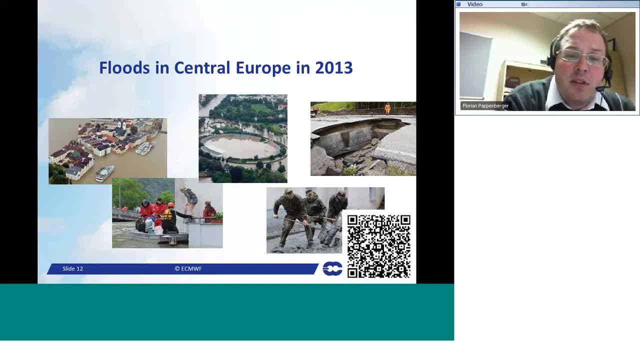 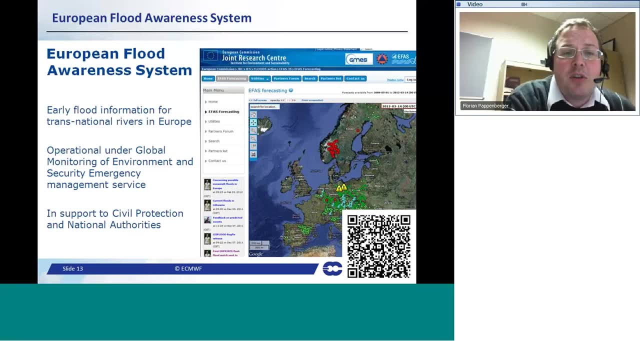 It's early information for transnational rivers, It's operated under Copernicus or GMES and it's in support of civil protection national authorities. And why do I talk about this? Simply because ETHNWF is the operational service, ETHNWF is the operational center of it, or the computational center of it. 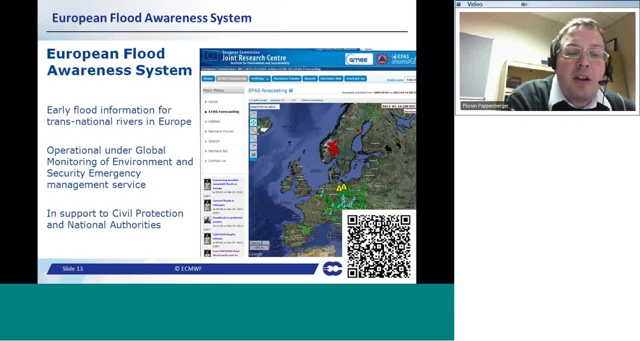 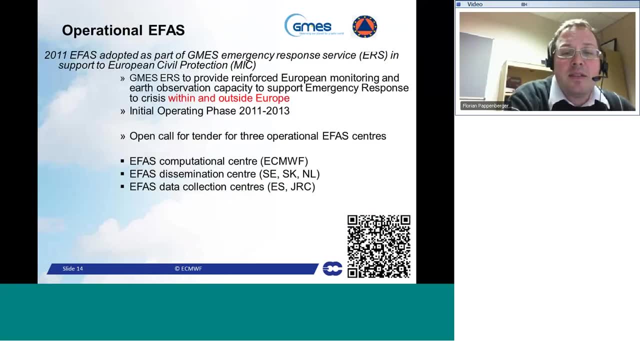 We are running the ETHNWF system here on a daily basis on behalf of the European Commission. There's all the other partners involved, For example SMHI. Slovakia and the Netherlands are the dissemination center. They do all the communication to the end users. 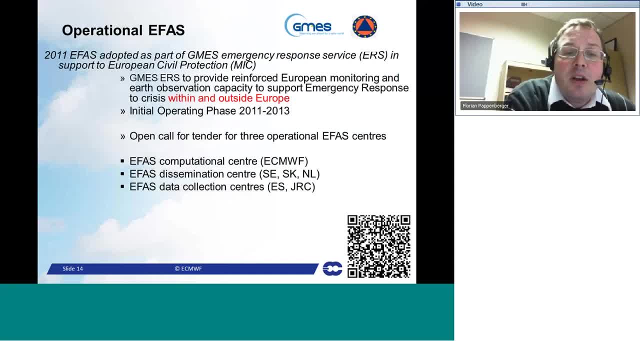 And then we've got a Spanish consortium which does hydrological data collection, And the JSE, the Tron Research Center of the European Commission, still does the metallurgical data collection, And that's the ETHNWF. It's a very important part of the ETHNWF system. So just to go back and try to remember, I know it's June 2013.. It's actually not that far away. Some of you may have forgotten. There was some persistent rain across Europe. It caused major flooding of central Europe. 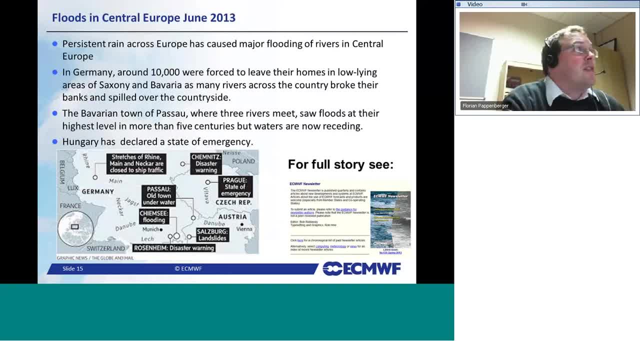 In Germany around 10,000 people were forced to leave their homes, particularly in Saxony-Bavaria. Bavaria is in the southern part of Germany, bordering Austria in the eastern part of Germany, bordering to the Czech Republic in Poland. 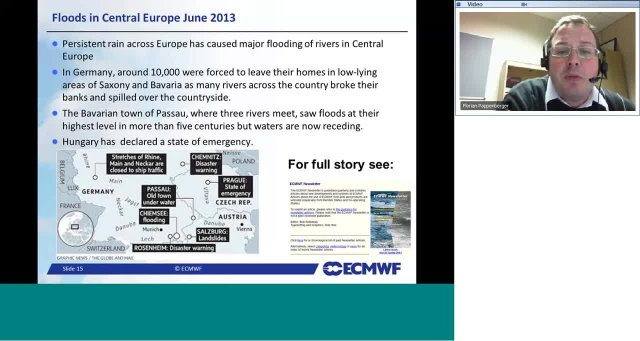 In particular, the Bavarian town of Pasa was hit very heavily and it saw the highest levels of flooding in more than five centuries. so we didn't have any of that earlier And at that particular stage Hungary had declared a state of emergency. 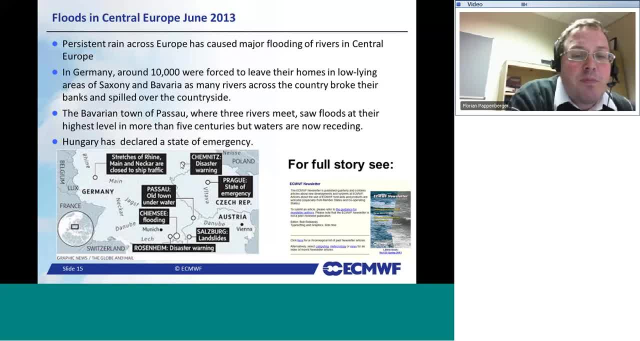 I'm going to show you a small subset. As I said, the full story is actually up here in the ESNWF newsletter, which you can look up, And there's also paper in HESS, an ideological journal by Günter Breschel, on that. 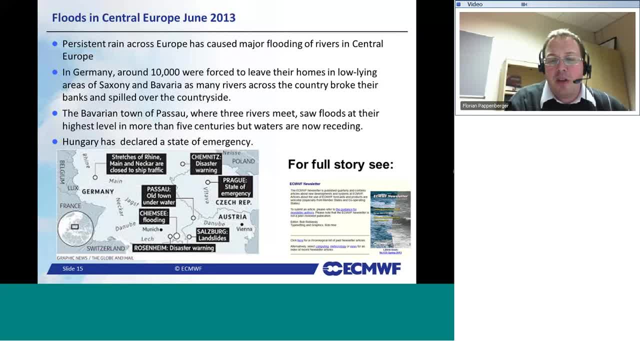 What type of flood warnings were issued or were in place in this particular case. You can see here quite nicely. all the triangles show you there was a flood warning. The orange triangles are alerts, the other one are warnings. don't worry too much about difference. 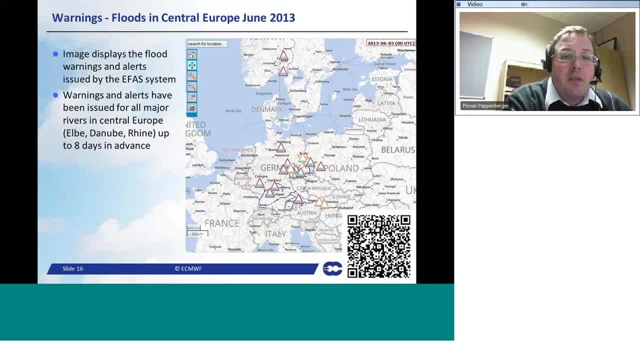 And, as you can see, it did hit more or less central Europe, large parts of Germany, parts of Poland, parts of Austria, parts of Hungary. Was it really an extreme? Well, if you just have a quick look at precipitation, then what we have here is the precipitation on the left-hand side. 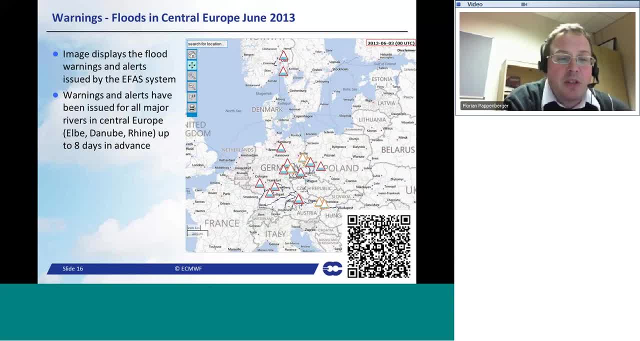 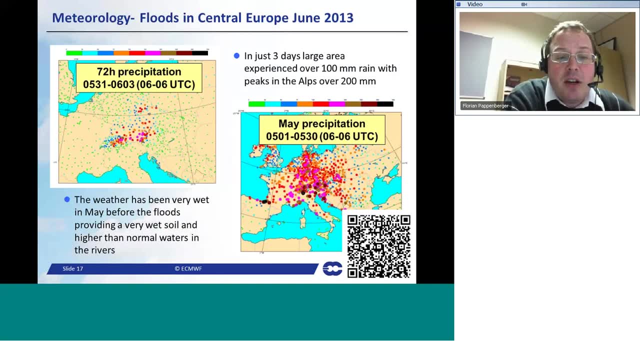 for the precipitation just before the event. so end of May, beginning of June, It goes from 0 to 0.6 to 0.6.. On the right-hand side you've got the average of this precipitation. The color scale is exactly the same. 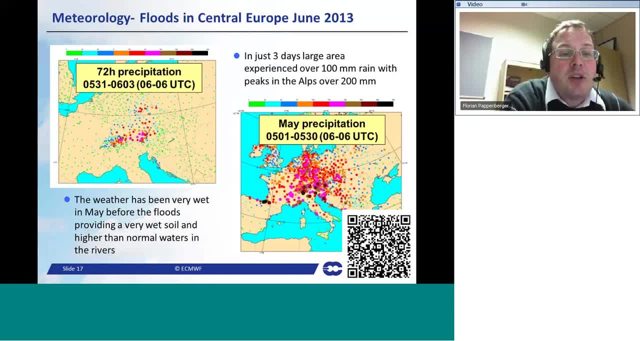 And in this particular event, in just three days a very large area was hit with 100 millimeters of rain, And somewhere in the Alps it even peaked at 200 millimeters. And this wasn't the only problem. The problem was also that particularly the month before was extremely wet. 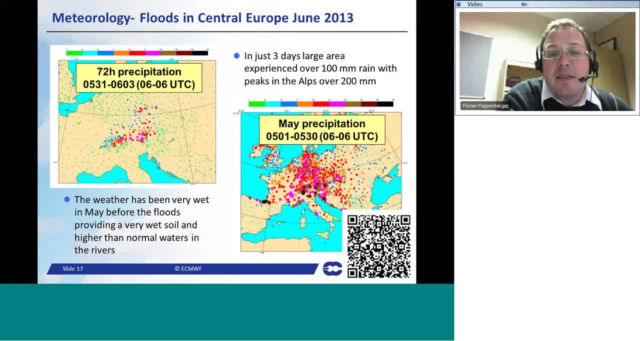 So the soils were wet and the river levels were actually higher. If you look at the deterministic forecast- something I don't do very often because I think some of the forecasts do tend to have a better skill base- On the right-bottom-hand side, you see the observations again. 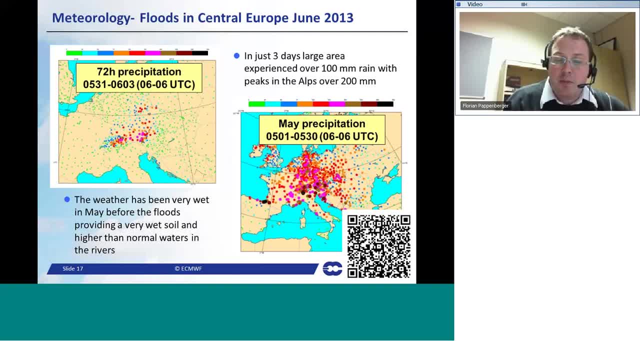 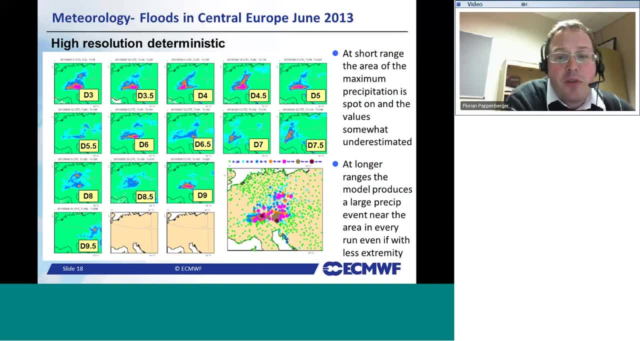 Just use it as a sort of indication here where you expect the event. Here you see different forecasts. You see forecasts coming out from ten and a half days to three days. Half days because ECW issues two forecasts, one at 0.0 and one at 12 UTC. 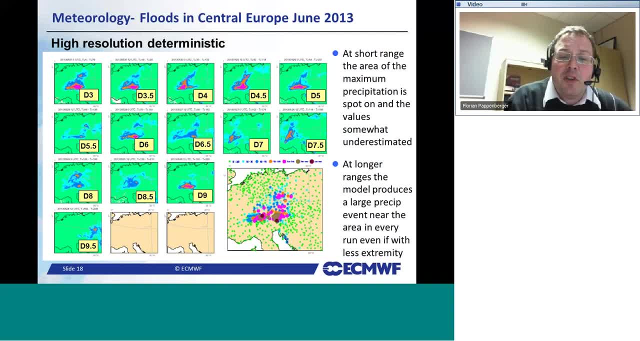 You can see that. You can see, in the beginning there was some sort of signal. In a way it's 70 hours accumulated precipitation which you see here At the short range. you can see that the precipitation becomes actually spot on. 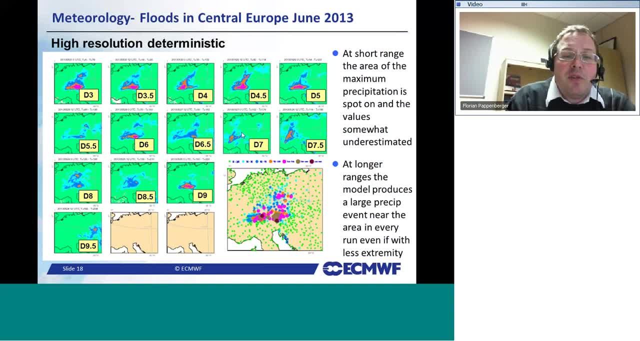 What you can't see that clearly is that the precipitation was severely underestimated. So although we had location extremely well predicted, we didn't have the magnitude very well predicted. In the longer range. you can see that precipitation always hit the right areas. This one, for example, is too far east, too far west. 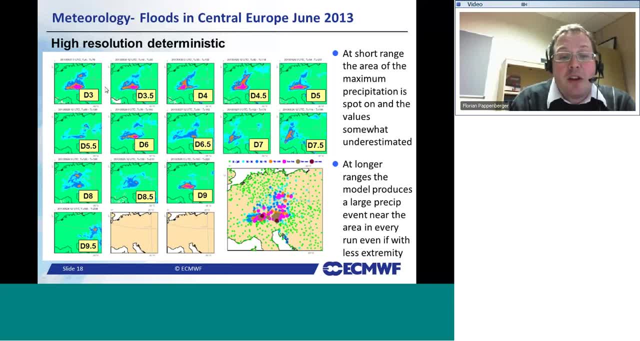 Here you seem to have a pattern which is much larger. In the day nine it seems to be roughly correct. So we did have some signal that there may be something coming in the area, but the location wasn't that well predicted. I already talked about the Extreme Forecast Index. 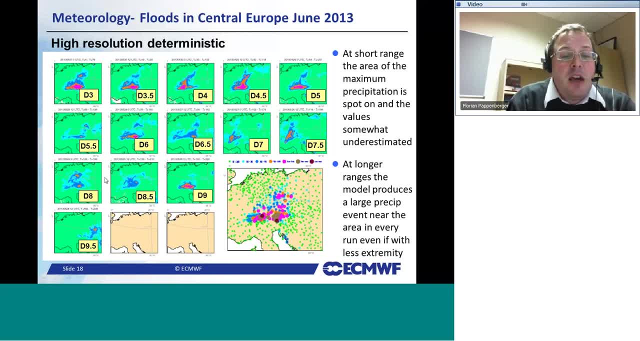 The Extreme Forecast Index gives an indication of how extreme the event is in comparison to climate. Here you've got Extreme Forecast Index. Here you've got Extreme Forecast Index starting at day nine going down to day one. The color scale is fairly simple. 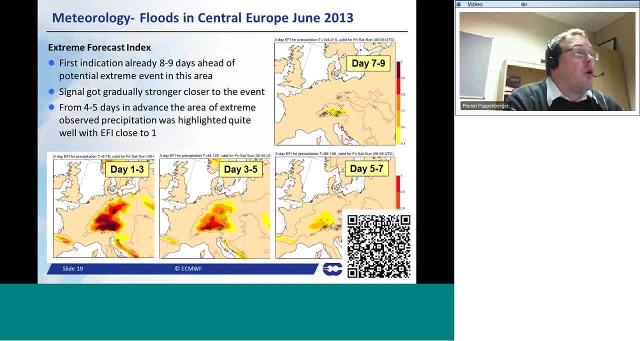 The more red the more severe it is. It's based on the ensemble forecast. You can see a very similar signal At day seven to nine. the signal wasn't very strong. The location was there. Day five and seven the signal became a bit stronger, but the location was probably a bit too far west. 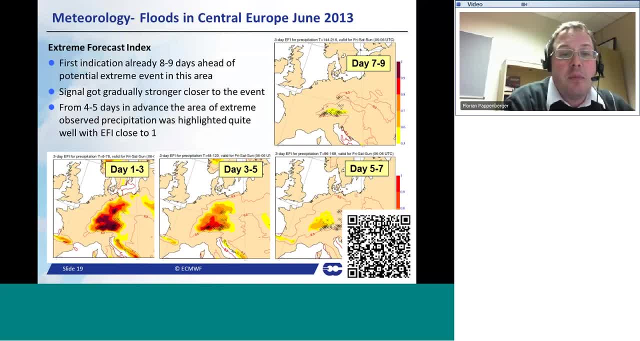 Day three and five and one and three, it's very clearly to be seen that there seems to be some really extreme precipitation coming along. So the forecast got gradually stronger the closer we got to the event. So far, the previous plot was based on precipitation at a point. 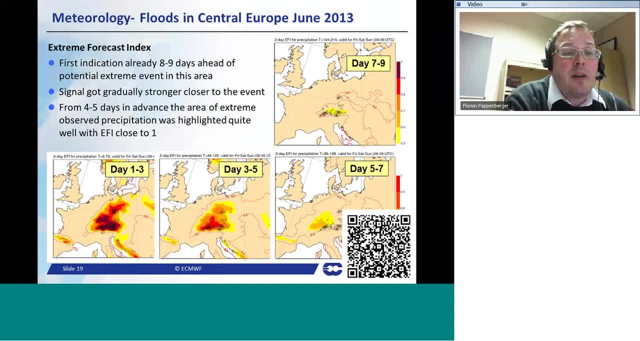 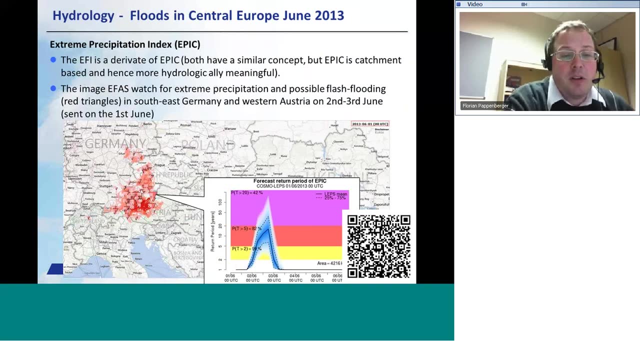 It's, of course, clear that the thing we are really interested in is actually precipitation over catchment, And for that we have developed something called the Extreme Precipitation Index, which accumulates precipitation across those catchments that are logically more meaningful, And we particularly use this for more flash flood forecasting. 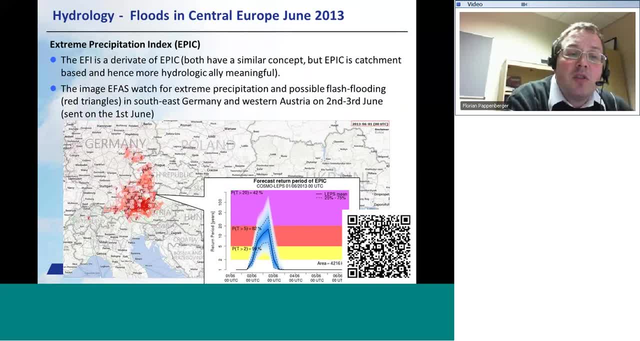 And what you see here is an example of extreme precipitation. The red triangles are possible flash flood warnings And you can see that the forecast is from the first of June, So it's a very short-term forecast, But you can see quite clearly. there was a clear indication that even on a catchment aggregated scale, 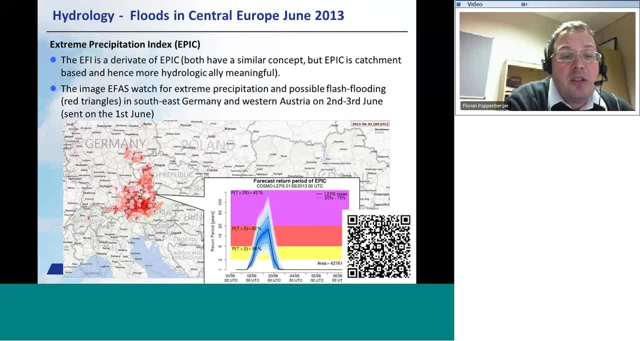 an extreme event was coming. Here you see one of the plots which I showed earlier, With the return periods here at the bottom. It's based on the CosmoLabs ensemble And you can see a large number of ensembles actually predicted fairly high return periods. 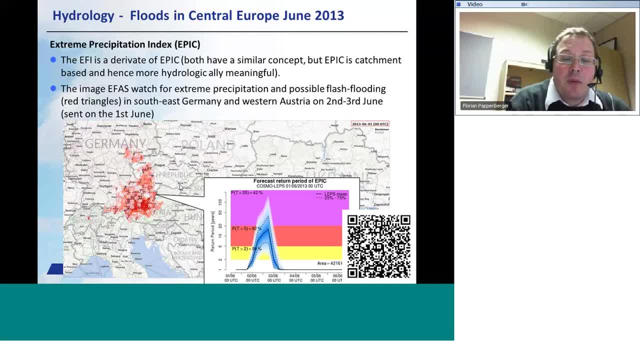 If you just look at the probabilities of the ensemble itself, So the ensemble forecasting And here the probability of exceeding 100 mm, We're starting at day 9 and going to day 1. again. There's a weak signal of 8 to 9 days in advance. 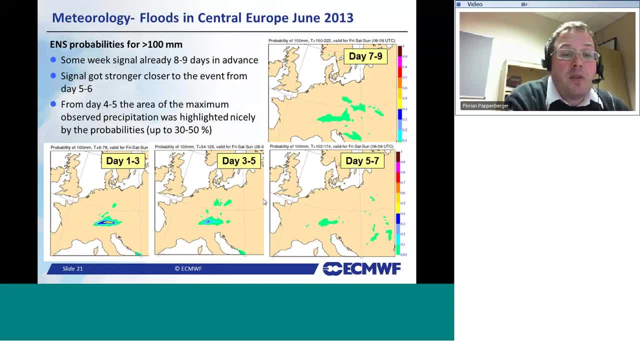 And I think one has to understand that 100 mm isn't happening very often. So if you see that type of signal already 8 to 9 days in advance, that's fairly interesting. Similar to the domestic forecast, the signal got stronger and stronger over the days. 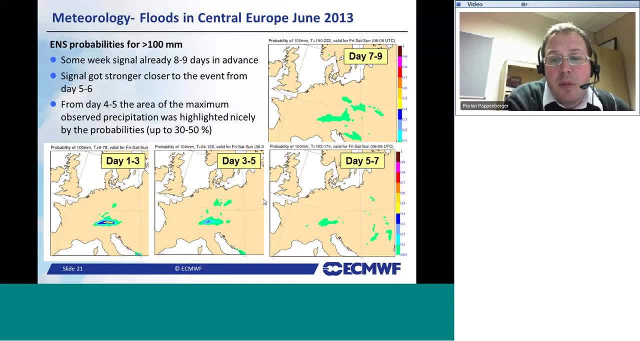 Particularly from day 5 to 6 onwards And then at day 4 to 5,. the area of maximum precipitation was extremely high And the probability of getting that extreme precipitation was extremely high. This is 100 mm. Don't forget I actually said that in the Alps. 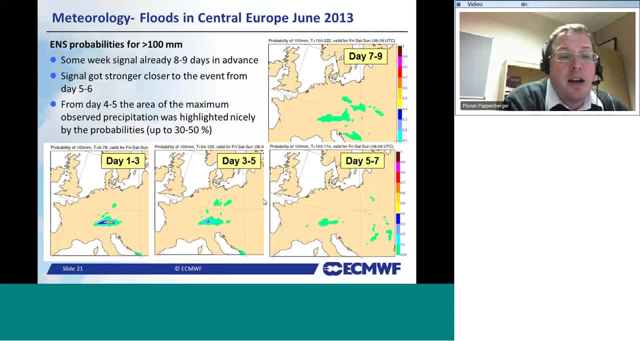 so this area where we actually predicted extreme precipitation, there was peak accumulation time, was actually 200 mm. Just to demonstrate you that actually the soil was very wet, And here we've got a picture of the OIMETSAT-8 soft product. 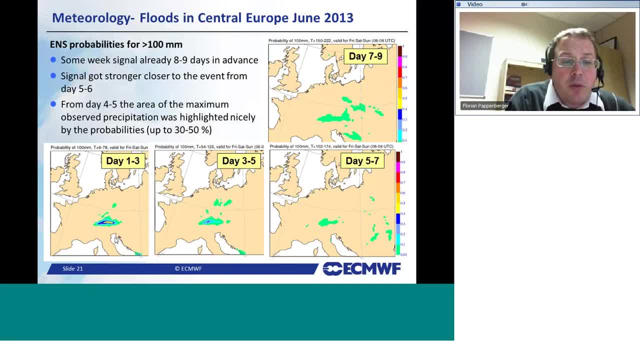 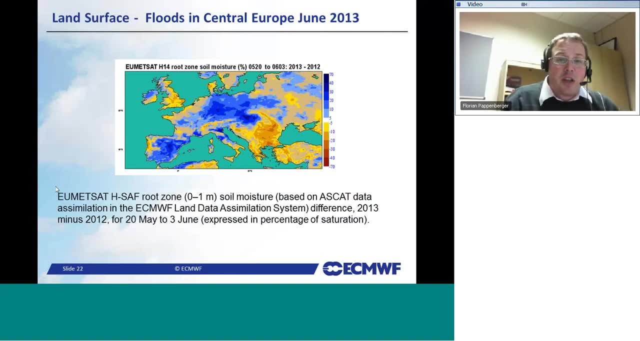 It's the roots on soil, moisture, space And ASCOT is also produced here at ECWS, And what you can here see is the distance from 2013 to 2017.. 13 to 2012 for that period at percentage of saturation. 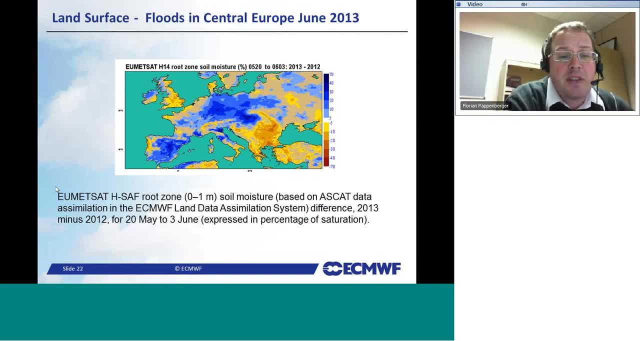 Everything which is blue is extremely saturated And you can see the soils were indeed extremely wet, So we could even observe from satellites it was wet soil. So we saw it in the metallurgical forecast, We saw it in precipitation forecast. We saw it in forecasts which were more tuned to hydrologist and catchment base. 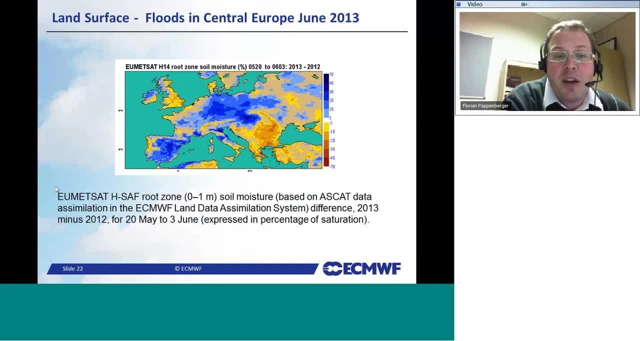 We saw it in our extreme forecast index. So did we also see it in the stream flow. And here you've got an image for the city of Kastel. I've just told you it actually did experience the flood level which wasn't observed for 500 years. 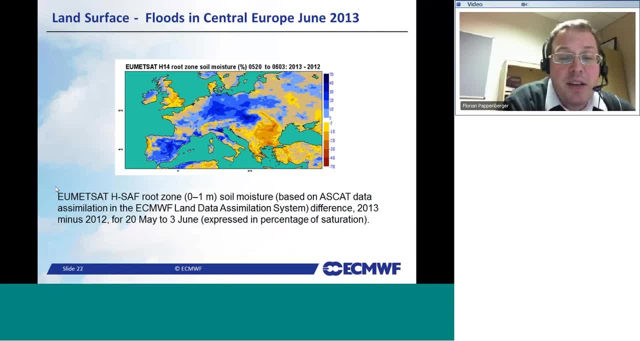 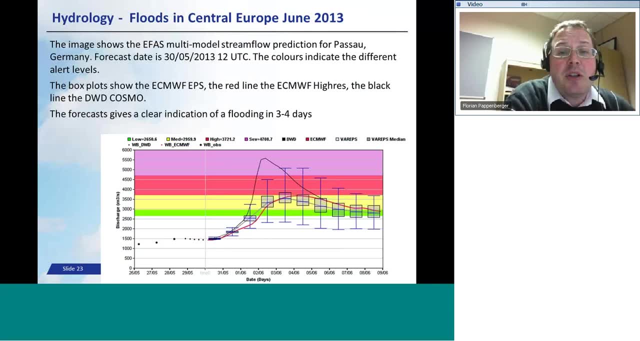 Here you've got a typical EFOS forecast plot. What you have is this chart: on the x-axis, You've got a date. on the y-axis, You've got the ensemble represented as box plots. The black line is the high resolution ECWS forecast. 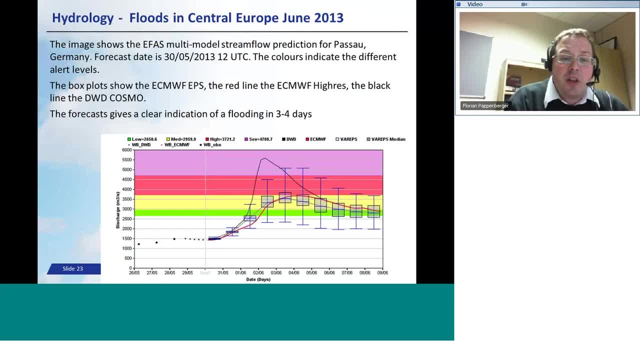 And the black line is the forecast for the general weather service. The red line is the high resolution forecast And you can see quite nicely that actually on the 29th we can see there's a certain peak appearing And the purple area which is the severe alert level. 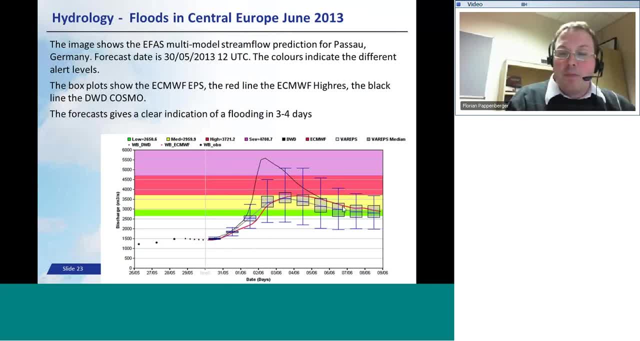 So we've got four different alert levels here was hit And there's some probability of it actually getting up to 5,500 to 6,000 cubic meters per second. It has to be said, I was completely underestimated. Discharges were far beyond 8, up to 10, even, some people estimate. 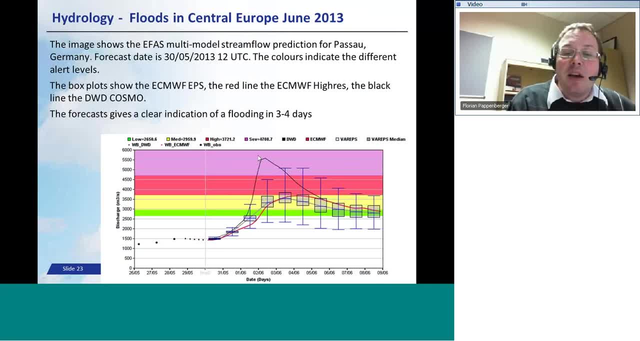 So although we predicted the extreme event, we didn't predict the severity even close If you look at this in a more historic time series. So the plot before was a single forecast of a single day. If you now have here forecast of different days, 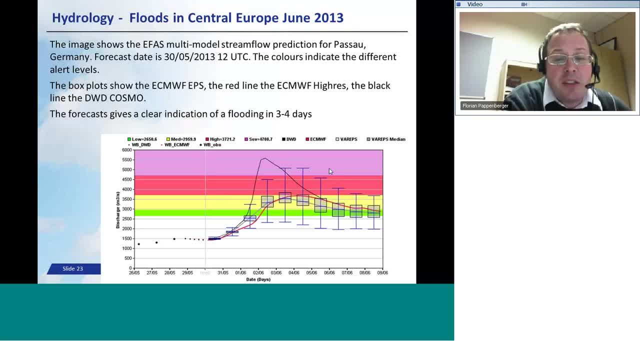 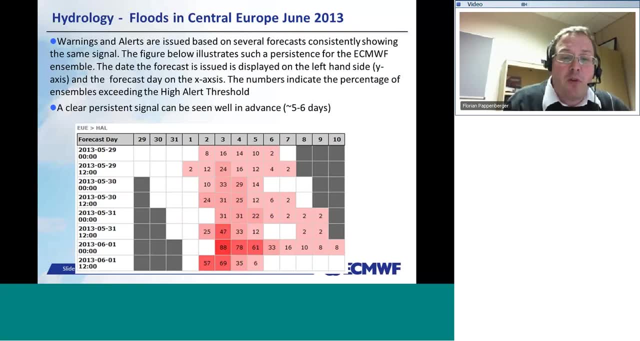 So we've got forecast issued on the 29th of May, on the 30th of May, 31st of May and 1st of June. You have here the percentage of Osombos exceeding the high alert level. So on the 29th of May there was the prediction that 8% of the Osombo members exceed the high alert level. 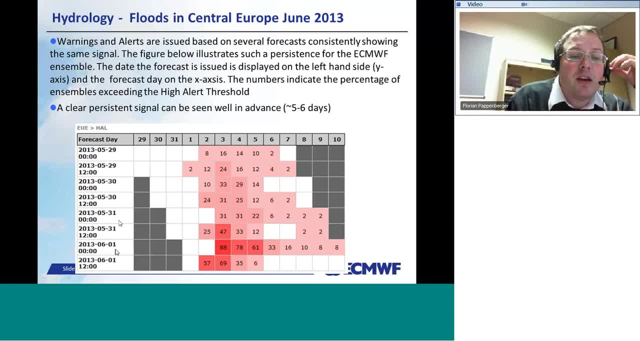 On the 29th of May for the traffic log forecast it was 12%. On the 30th it was 10% and 24%. This plot illustrates quite nicely that actually it was a very persistent signal five days ago, Five days in advance in the European flooding. 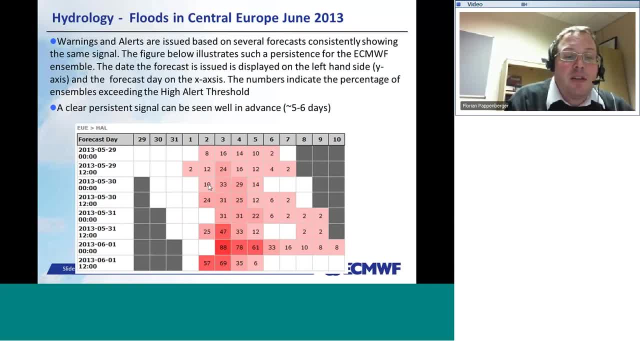 So there was a certain signal coming up. As I said, severity was underestimated, But it was very clear that we had a signal reoccurring that the forecast would be getting worse. Do you see with me? showing these plots is always that. I'm showing you single case studies. 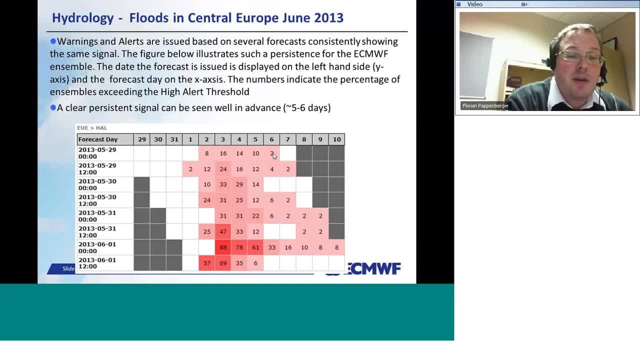 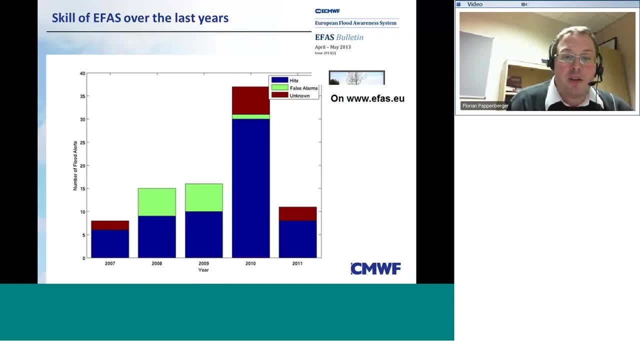 I'm showing you a single example. This is not very good enough for verification. This is a number of verification or very simplistic verification for the European flood awareness. We've got this system in the last years. We've got simply here the list of the hit falls and alarms of the unknowns. 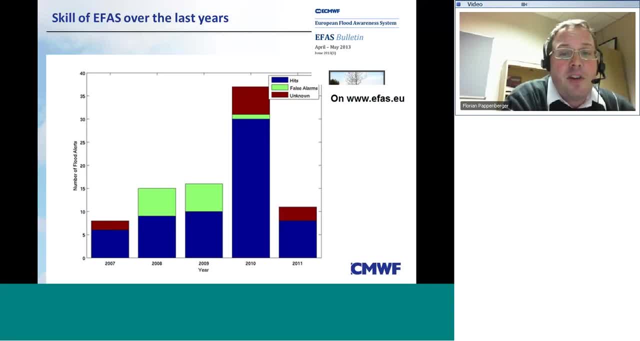 So how often were we right in terms of our forecast? I only have it up to 2011 on this particular plot. If you want to see the rest, we've got to publish a monthly, a bimonthly bulletin, Which you can find on eHearteu, where we report our past performance constantly. 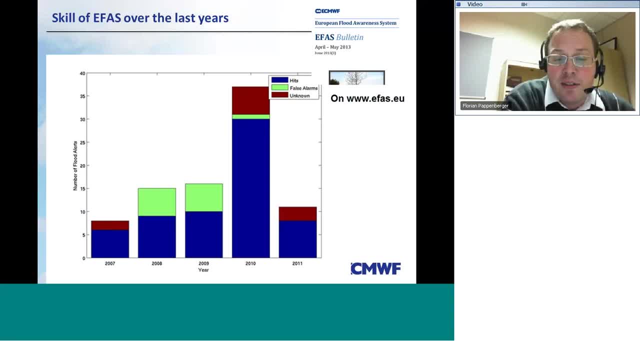 But what this plot quite nicely illustrates is actually: on average, we have been better in flood forecasting, so we have more hits than false alarms or unknowns. and we can also show this in other skill scores and more complicated settings. but actually this forecast system is skillful. it's not just that single case study which works. 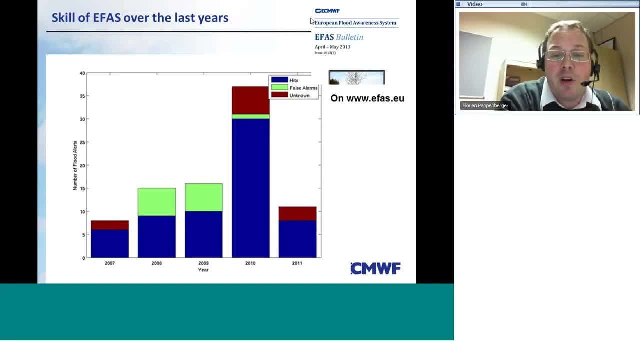 This led us to the development of a global flood awareness system. So far, we've only covered the European continent, so that tiny part here of the world, but we decided to go ahead and see whether we can do this also on a global scale. and here is. 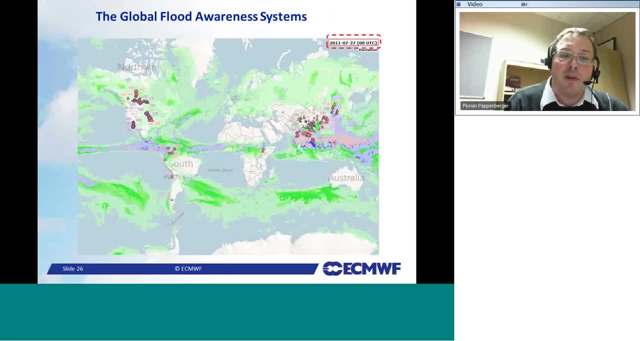 the screenshot of the global flood alert level system from the 27th of July. You can see the type of forecast we've produced, very similar to the ones before. we've got here the discharge we have here the asombles. this time they're more indicated as blue lines. 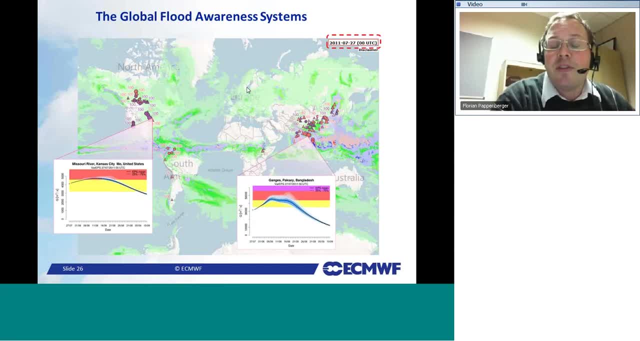 and we've got, as you can see here in the Ganges and Bangladesh, different alert levels. The triangles indicate regions where our system suggests that you have a look, we have some sort of data. This is an automatic way of trying to raise awareness, because it's impossible for a forecaster. 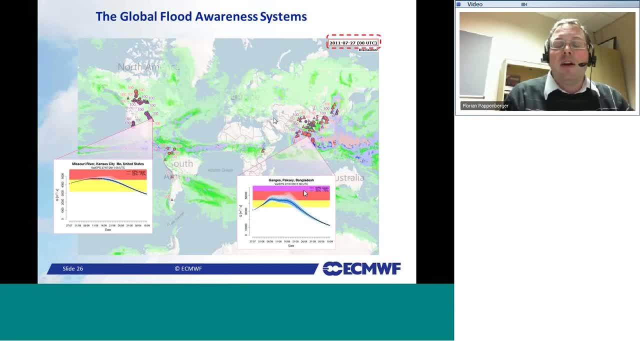 on that scale to look at every single point and what you can see quite nicely. the triangles are quite good distributed and you can click on the individual triangles and get these discharge hydrographs Overlaying. you've got the probability of precipitation. so just so you have an idea of where the precipitation. 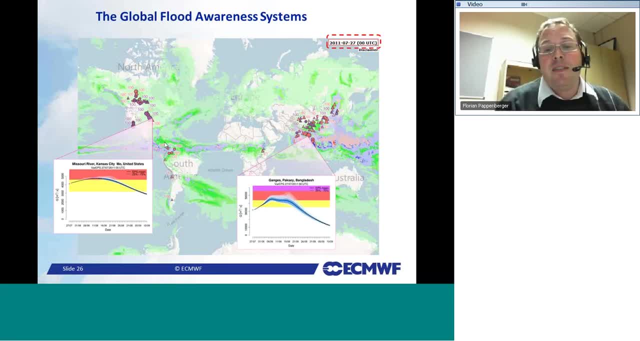 was predicted to. The system is fairly simple. It couples the EZWF land surface model, called HTSL, to the list flood running routing model from the JSC. it's a collaboration with the JSC. I believe it's probably the future. it's the first integration of, or the first full integration. 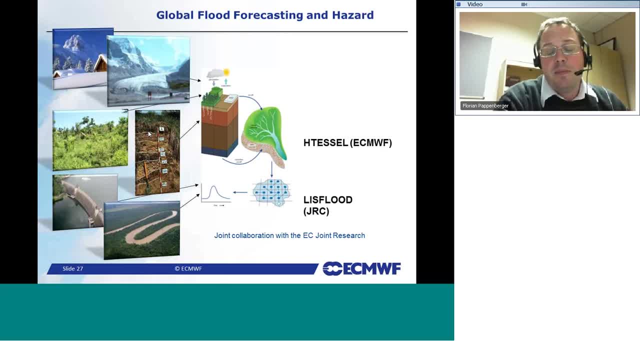 of such forecasting system into the American Weather Prediction Model or into a land surface model. As I said, we've done some more detailed skill analysis and I'm only going to show this plot. Next year, Lorenzo Alcieri will be presenting this. 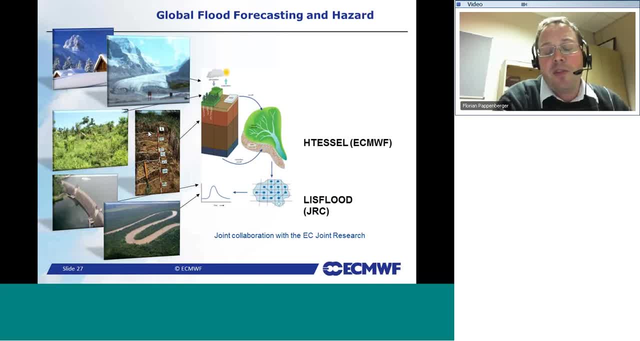 Next year Lorenzo Alcieri will be presenting this. Next year Lorenzo Alcieri will be presenting this. My colleague Andrew Kohn will get for that and he will go far more in depth into that one. And here I show the performance of our sample forecasts using the shear PFS. 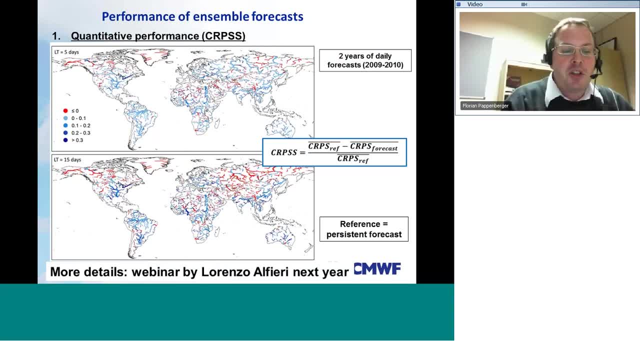 Very simple: Everything which is red, nothing more skilled. Everything which is blue, have skill And here for a lead time of five days from the lead time of 15 days, and you can quite nicely see that there's more blue than red, which is encouraging. 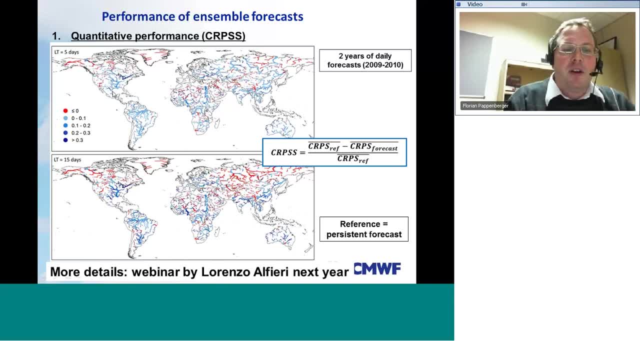 They're not very good anywhere. There are certain regions, particularly where we have uncomfortable pursuant to theкраiliar Spaceage. This is what it is going to look like Here. we're not very good everywhere- snow, melt, issues which are red, so we're not doing that well, but large parts of the globe. 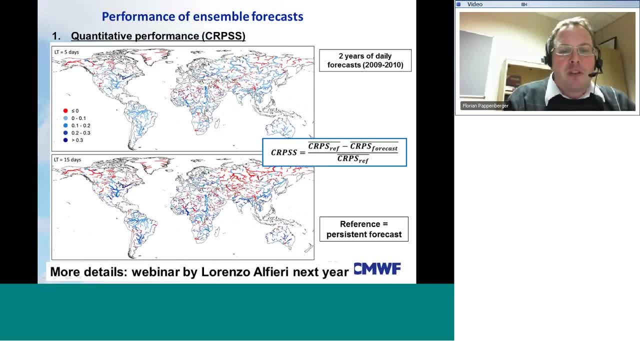 are blue, And then, if you go to 15 days, of course the scale deteriorates. we still have skillful forecasts in large parts of the globe, but many parts of the globe also have no scale. And then, of course, it's very interesting because it gives us the motivation to try to develop. 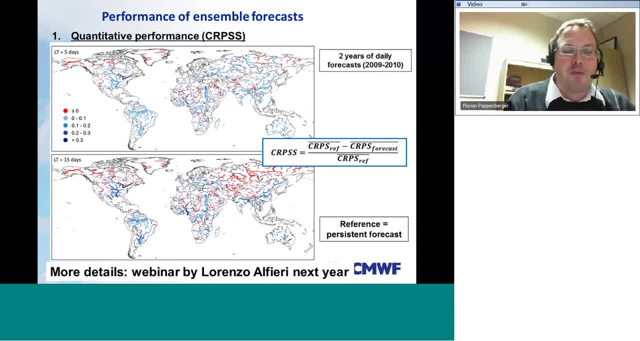 the system further and actually getting better. So far I've talked about medium range forecasts and I'm going to now quickly skip into seasonal forecasting and drought forecasting. I think it's always interesting that we cover the medium range, but I think you shouldn't. 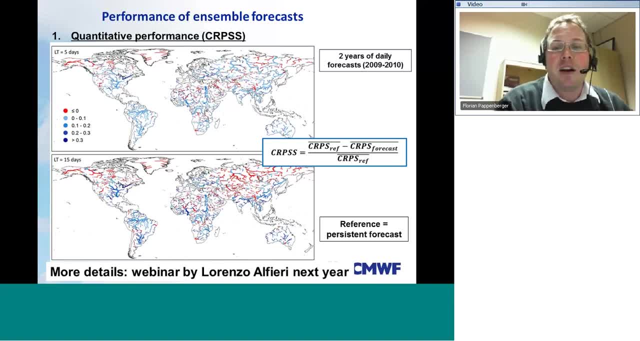 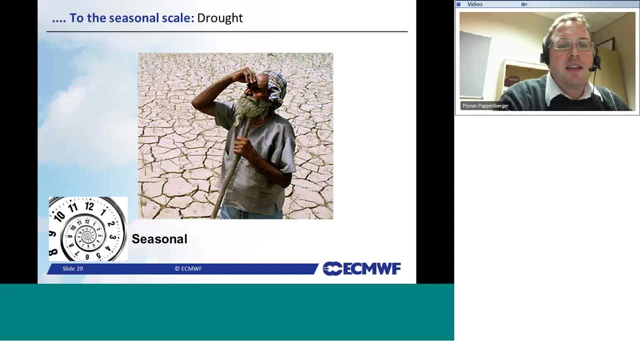 forget that many hydrological applications and many water resource applications are also fairly important on the seasonal scale or need the seasonal scale. I'm not trying to replace any other systems. there's many other systems out there and I've just brought in the two US ones: the US Jout Monitor, US Seasonal Jout Outlook and the 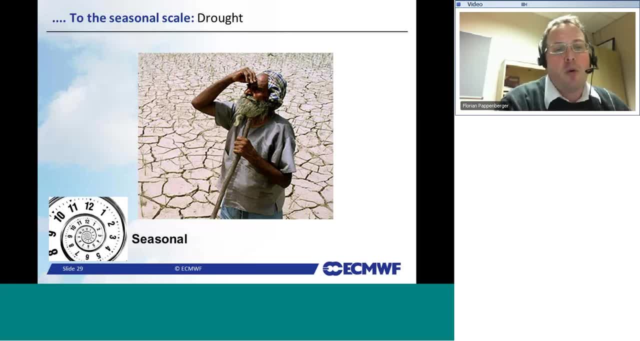 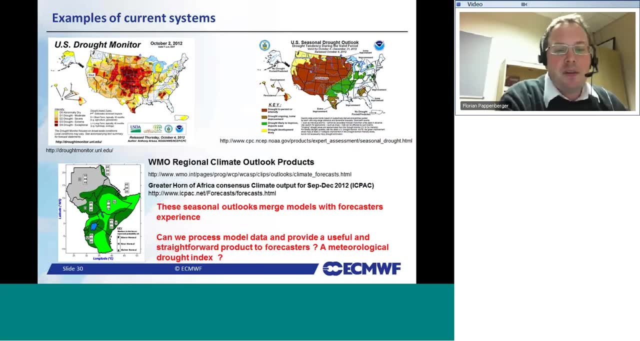 US Water Monitor, There's Greater Horn of Africa, Consensus, Climate Outputs and so forth. Our interest here was really more. can we use ESMWF forecasts to do this type of analysis and this type of forecasts? One thing one has to recognize is probably observations in terms of drought forecasting. 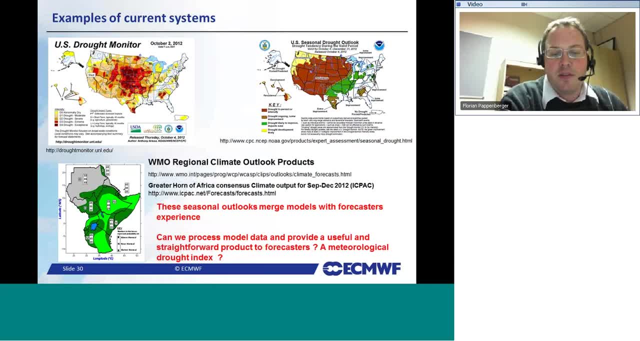 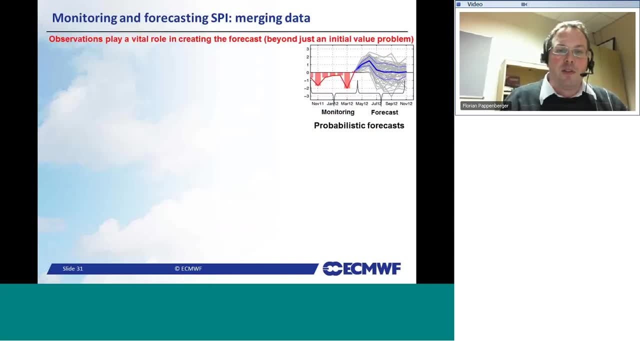 are far more important than they are in, maybe, flat forecasting, And the reason is that usually one accumulates over larger times. So I've given you a few examples: A precipitation anomaly or the standard precipitation index, which is in fact a precipitation anomaly. 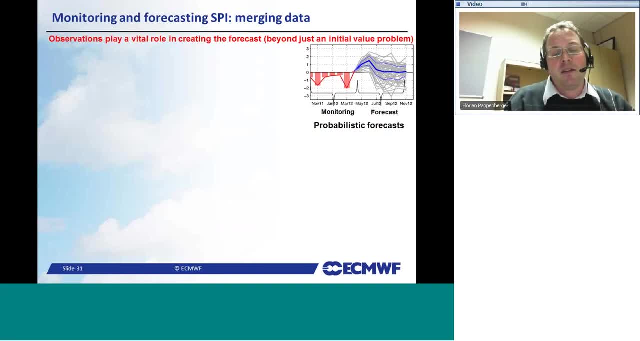 is always calculated over a certain accumulation time. So what we have here is a 12-month accumulation time, and if I want to do a forecast of six months, that means I need six months of observations and six months of forecasts. If I want to have a two-month forecast, I need eight months of observations and two. 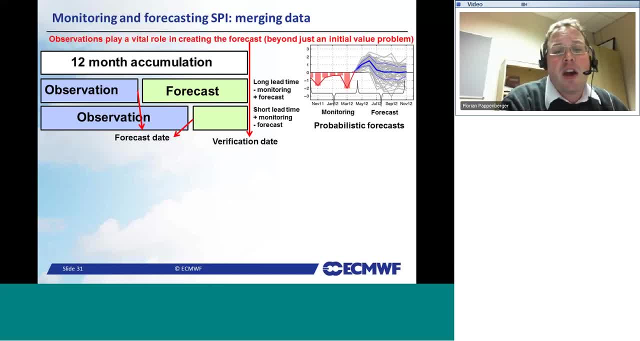 months of forecasts, So you can see that actually fork observations start to play an absolutely vital and important role. Of course, I also do spatial averaging over certain regions and I need to merge monitoring and forecasting, as I just mentioned Up here. you've got an example of that. 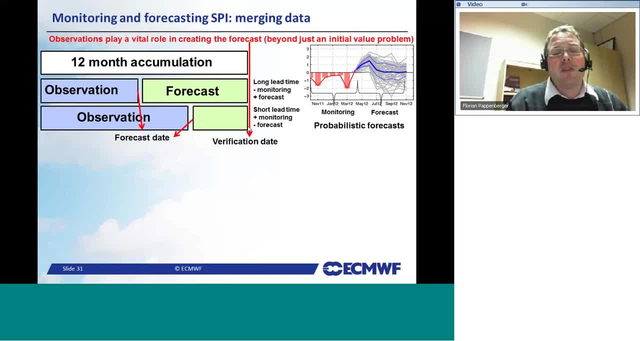 You've got a monitoring area. We have observed precipitation And then an ensemble seasonal forecast here, which is then the forecast. What I've shown you in the block before is a very deterministic view of the entire setting. I see the observations in a single block and I'm happily prepared to do this. 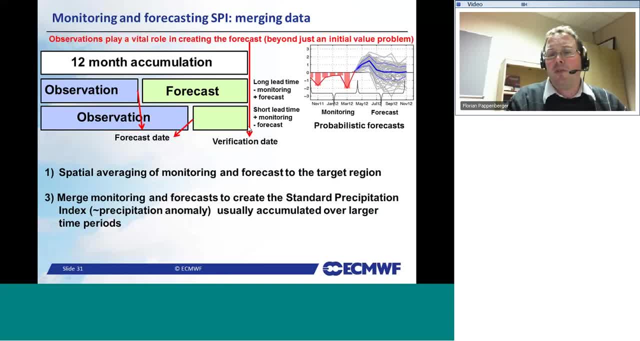 I'm happy, prepared to do the ensembles or the uncertainty in the forecast. What we shouldn't forget is that very often actually, we've got no real clue what the observations are. So even observations in large parts of the globe have a large uncertainty. 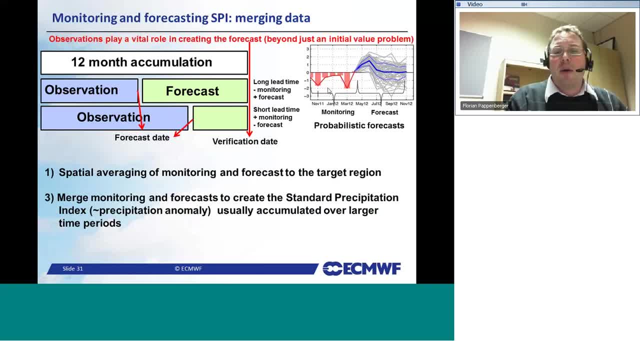 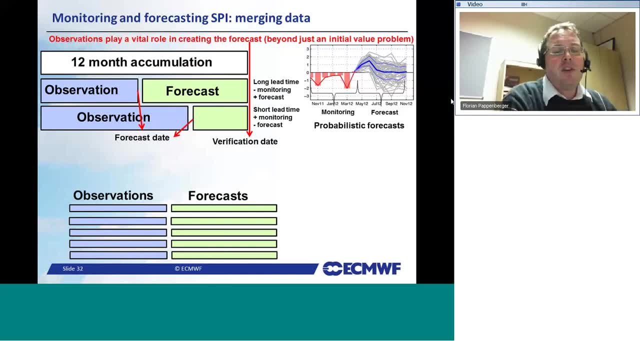 So I think we should recognize this and rather than just having a forecast ensemble, we should also have an observational ensemble. This could be seen as a double ensemble approach but actually recognizes the uncertainty observations. We do this in hydrology otherwise quite often. 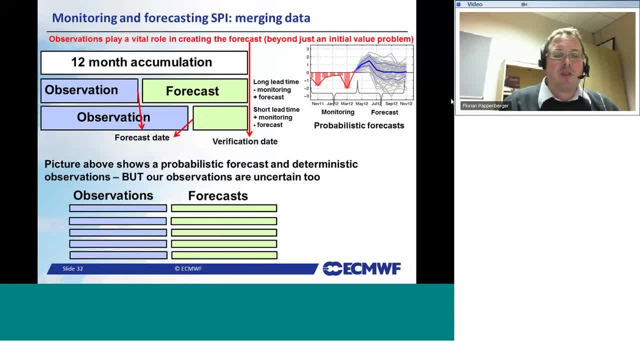 We do, I'm sorry We do uncertainty- initial conditions for many flood forecasting models. We do uncertainties in parameters. We do uncertainties in driving data, Particularly in the area of giant forecasting this becomes wider. to recognize. A simple example: here I'm showing you the probabilistic precipitation over the whole of Africa. 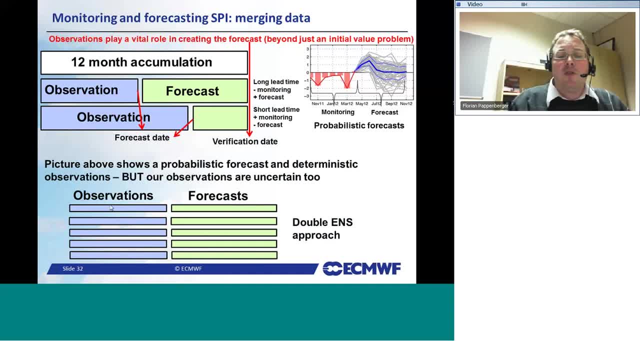 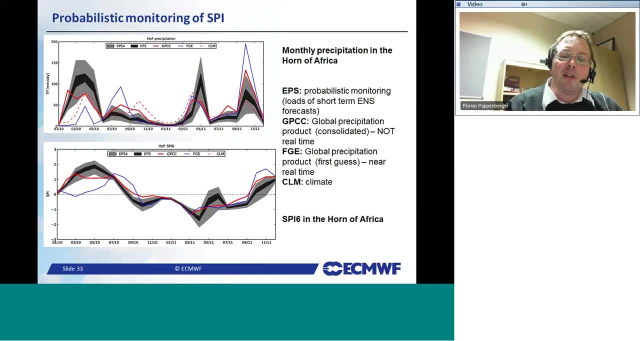 This is taken from a paper by Manuel Dutra which currently is to appear in the hydrological enhanced very soon. You have here different products. You've got your ensemble system Here in gray, the uncertain ensemble system. What we basically do? we string together a large number of short-term forecasts to build. 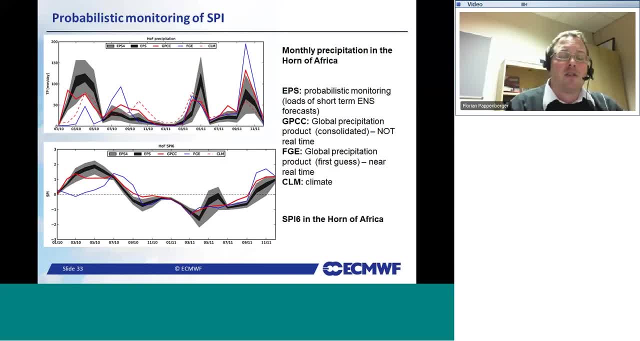 up a month. You see the monthly means here. You see the GPCP, which is one of the type of global observation products. Unfortunately they're not available in real time, so also they have a first-guess product which is FGE. 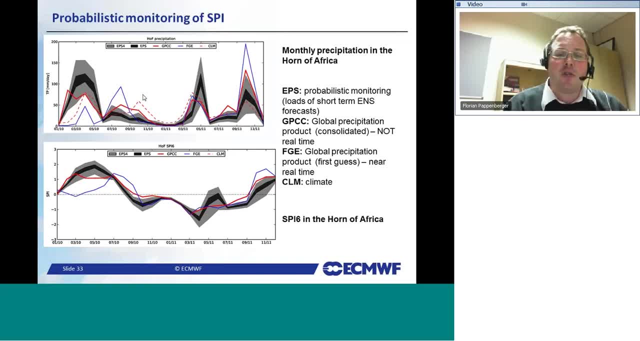 And we see the climatology And what you can see quite nicely is, even if you take GPCP as truth, we actually have to recognize the uncertainty to have the truth within our bandwidth, within our uncertainty bandwidth. Here's precipitation. You can also compute the anomaly here which is the SPI, so the standard precipitation. 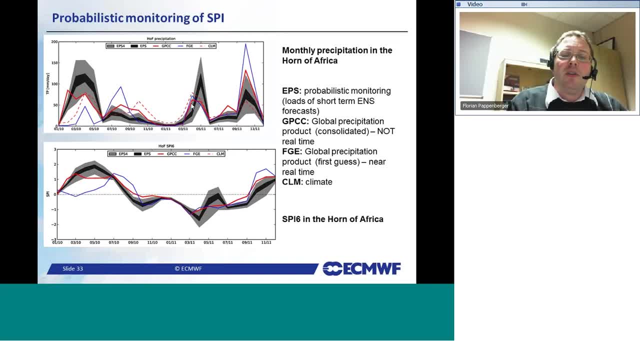 index again for the whole of Africa, And you can see quite nicely, maybe using just the first guess, it's not sufficient to represent the initial state for the seasonal forecast. You can even look into this even a bit further. If you look at loads of other type of forecasts, you can see that the initial state for the 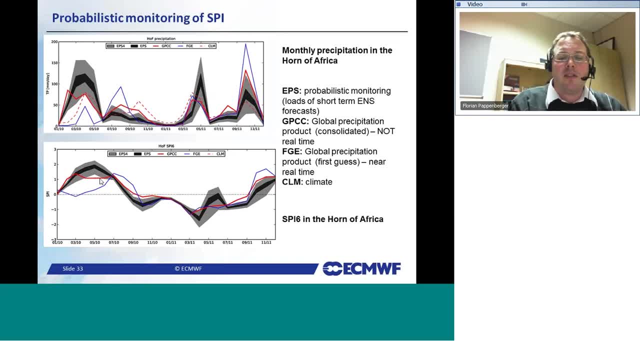 seasonal forecast. You can even look into this even a bit further. You can see that the initial state for the seasonal forecast. You can even look into this even a bit further. You can even look into this even a bit further. You can even look into this even a bit further. 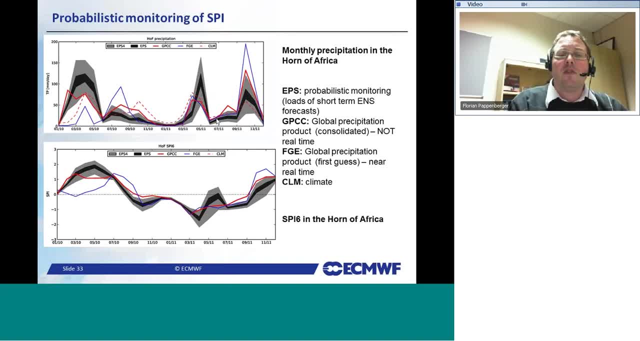 And you can see that the other type of precipitation products- and you have here also DRM, already converted into SPIs and precipitation anomalies. And if you look at correlations you can see sometimes the correlations are high, sometimes the correlations are not so high. 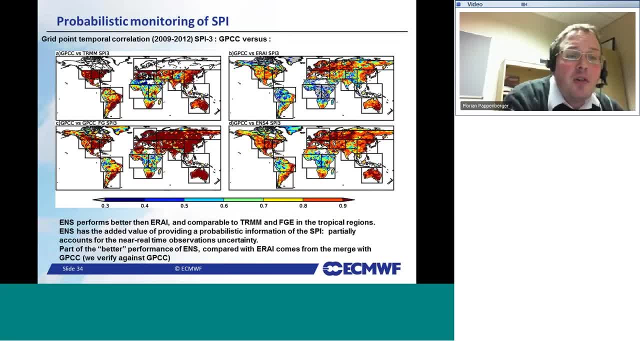 It's very clear that different types of products will have different type of information. We believe that the ensemble shows here that it's actually performing better than error intrain, in particular when it's comparable to DRM, which is here used as a ground truth. 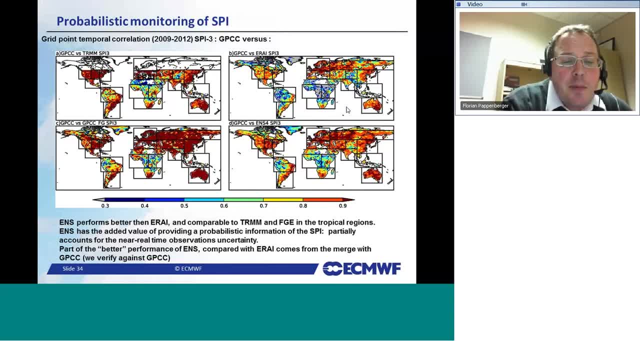 or the first guess, particularly topical regions. the ensemble has added value because probabilistic rather than just a debilistic presentation. So far I've talked about monitoring, similar to before, where I talked about climatology. I didn't talk about forecasting. 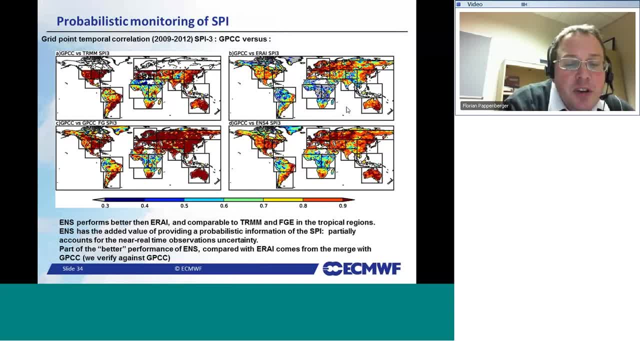 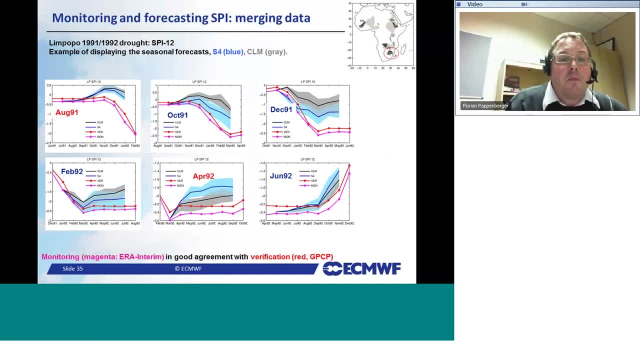 Of course I've showed you forecasts before. this is just a quick sample, more or less, to round up the issue of forecasting of droughts. So forecasting, here again, the SPI, so standard presentation index, presentation anomaly: The lower the anomaly is, the higher is the drought or the more severe is the drought. 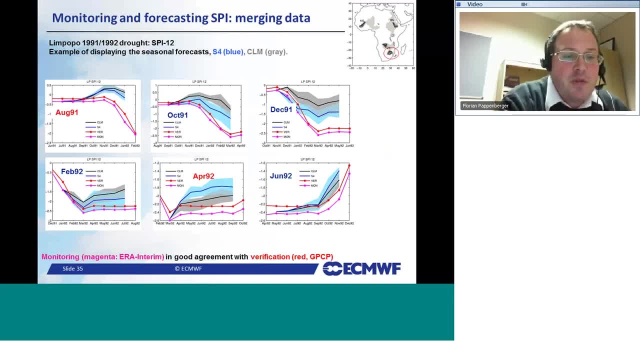 So if you're down here in the area of minus 1 to minus 2 or minus 0.8 to minus 2, we could see this as a sort of drought. and here you've got two different, you've got a forecast which. 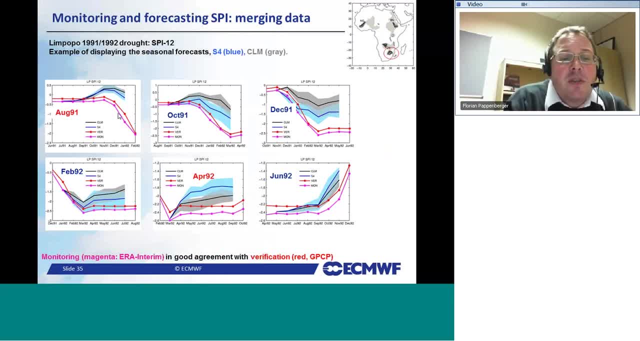 concentrates on the Limpopo in 1991-1992, the accumulated presentation over 12 months. the use of seasonal forecasting. So you can see, here we've got a forecast which concentrates on the Limpopo in 1991-1992, the 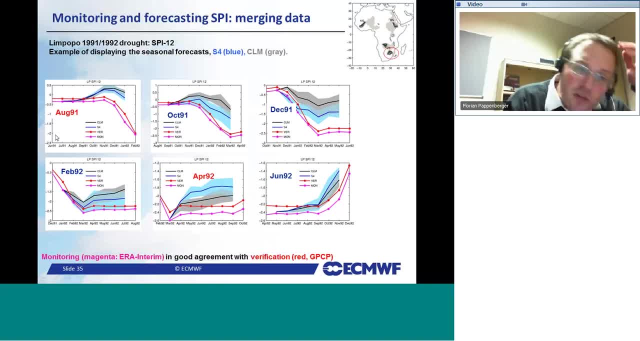 use of seasonal forecasting. So you can see, here we have a forecast in blue and also the climatology of what we would have observed, You see quite nicely, is two different types of observations which we've got here In monitoring is sort of the mage direito of the area, interim, the GPCP, the global presentation. 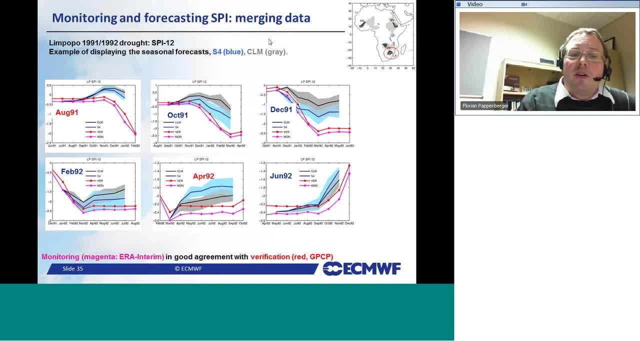 product is made, they quite nicely. we go through the months and we start October-August 91, October December, February, April, June. so we get closer and closer to the event in the observations. a drift into a drought situation here. 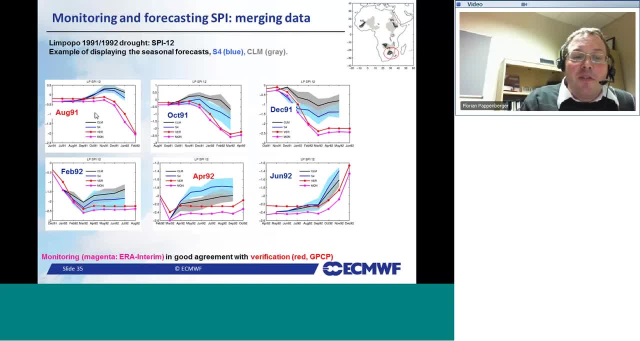 So the red and magenta line are under 2, under minus 1.8. And some of the forecasts, like for example this October one, indicated a drought. In a way it indicated that actually the forecast would indicate a drought in comparison to climatology. 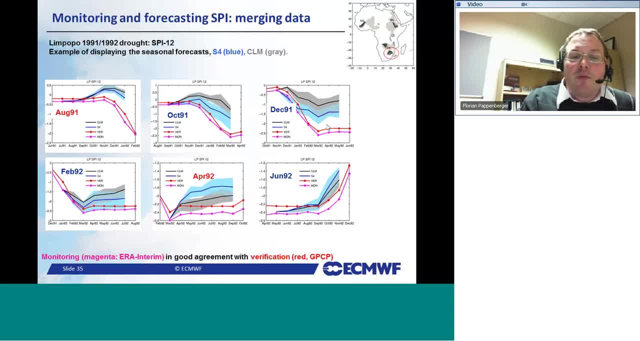 In other years, climatology was either comparable, like here in August, or another month, either comparable, like in August, a very similar forecast or maybe even a bit better than the forecast. So seasonal forecasts, in particular for regions in Africa, are not always the truth. 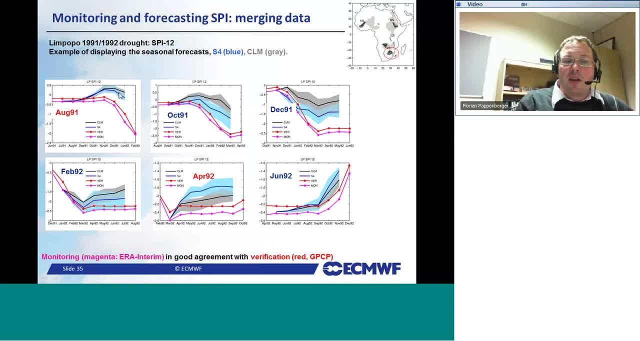 There's always also climatology and of course they have problems and errors. What we can say is that, although analysis has been done so far across the globe that, on average, with a seasonal forecast, you can be better in climatology and you're never worse. 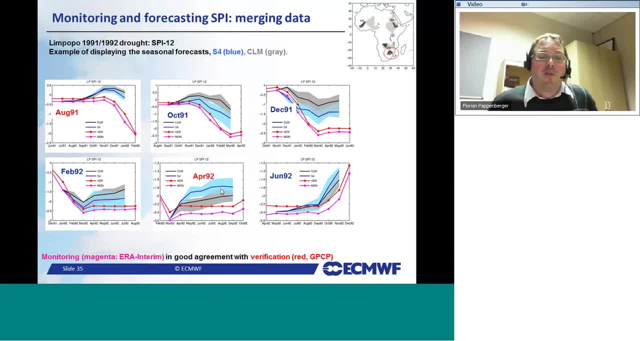 So you're better off in actually using seasonal forecasts rather than not using it. Just a simple example: here is the Oman of Africa, and this is taken from a paper from Emma, who is currently, who was visiting ECWF and is currently at ECWF again. 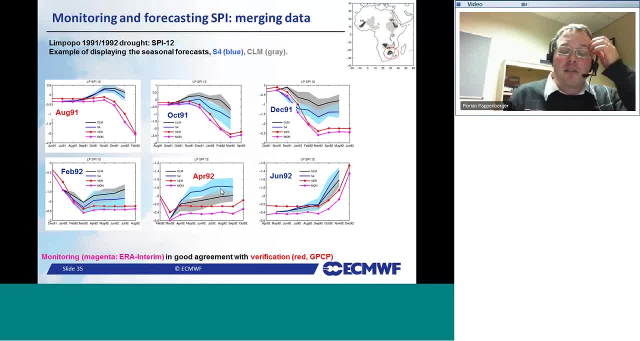 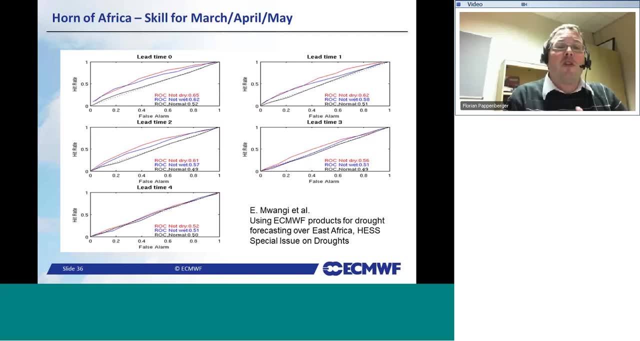 and she's also published a paper on that in HESS, on using ECWF products for a very practical application. So using these forecasts really for on-the-ground forecasting, and what you here see is the ROC score Every time you're above this black line. the ROC score is skillful, so it's better than 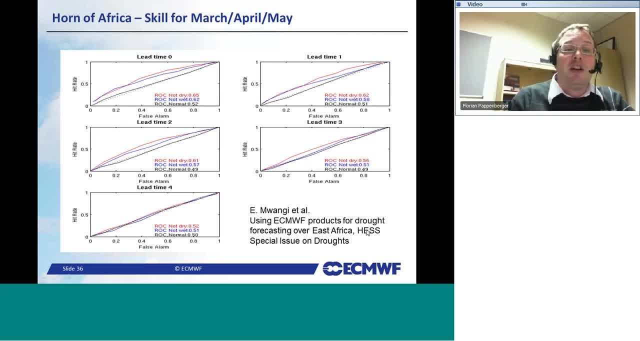 it's called skillful. We're only looking at March, April and May. Of course, depending on the season, you may have different skills. We're predicting two different events here. We're predicting you're not dry and not wet. You can see at lead time one, we are clearly above. 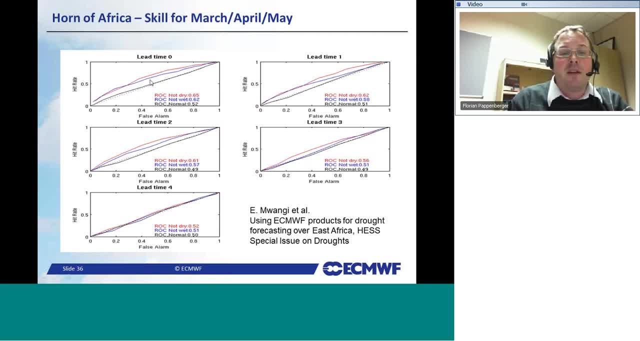 Lead time two, we are still clearly above, And lead time three and four we actually don't have necessarily that much skill anymore. So the seasonal forecast for the Oman of Africa for this particular season can be skillful up to lead time three If you look at different seasons. as I mentioned before, this is not always necessarily the case. 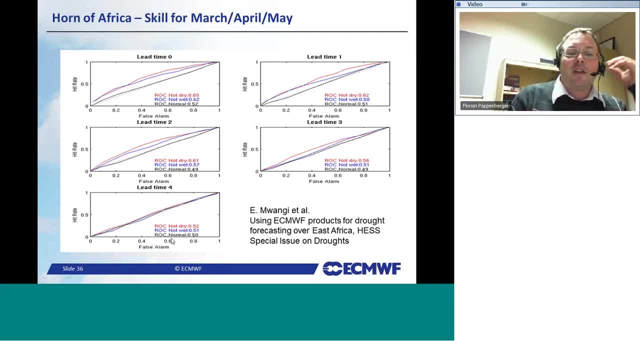 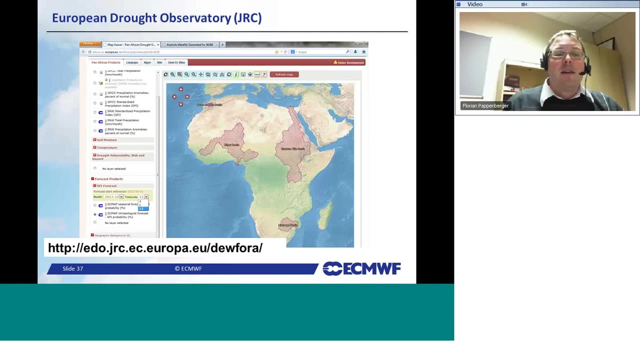 I already mentioned that Emma actually used this data and tried to demonstrate it on a practical example. We've recently been involved in the FORA project and in there we were also quite concerned that actually our forecasts are used. And here's an example which is on Africa, trying to integrate ECMWS forecast data. 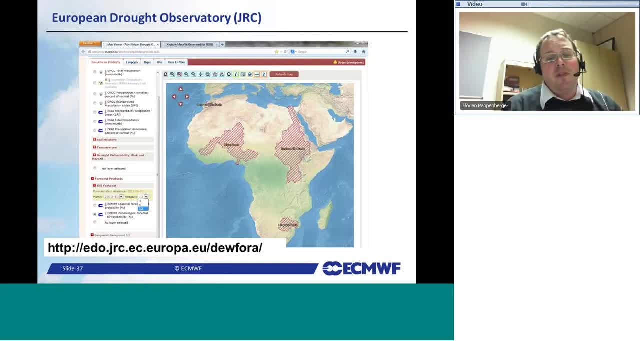 as well as GPCT and many others, in a forecasting system. I always quite like this slide because I find it quite ironic. it's done within a European child observancy framework from the Joint Research Centre in Asia-Africa, So it's quite nice. We have different test bases here, which you see here. 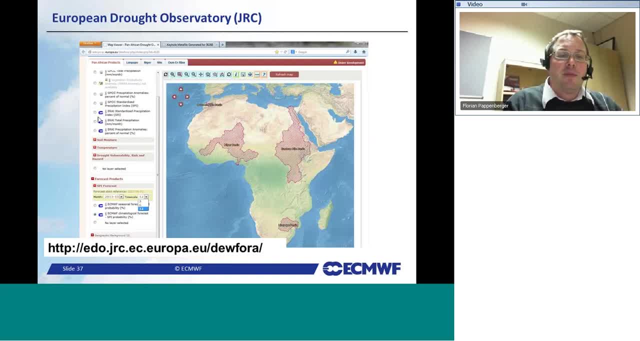 But you can actually go to this website and you can have a look and see how ECMWS forecasts compare to maybe climatology, maybe GPCT, and how what we would predict in terms of drought forecast. So I encourage you to have a look at the website. It's also very well documented to have a look. 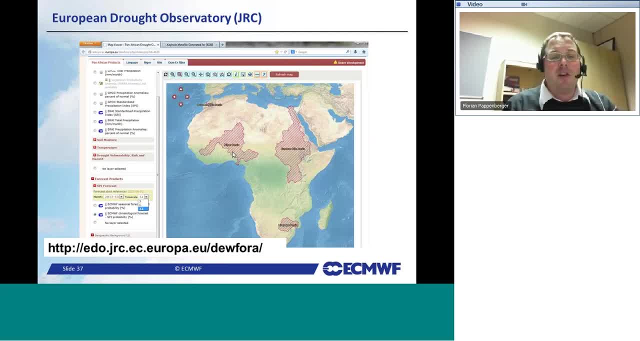 I want to very quickly make a link in my last five minutes, three minutes, in my link to climate In particular, because Tesla Visenius is going to give a webinar next week, next year about this: How to see the forecast and climate link. 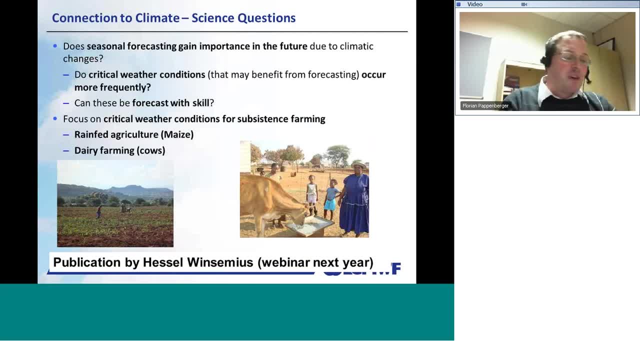 And I think we can make a link in the sense of: does seasonal forecast, is seasonal forecasting something which can be used in an adaptation strategy? Can we use it for something where maybe climate change may occur or may not occur? So the first question we have to ask is: does a certain critical weather condition occur more frequently in the future? 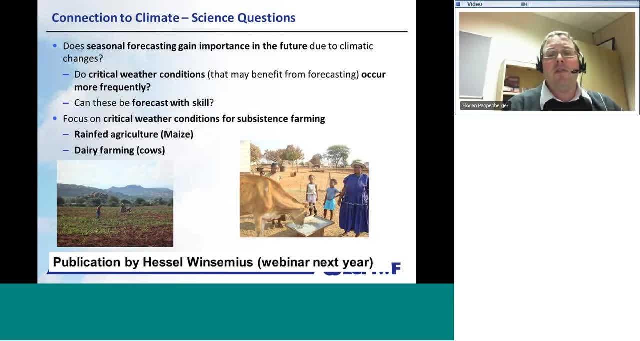 and can we forecast it on the scale And we predict when we can predict it? We can answer both questions with yes. Then we know that forecasting, or seasonal forecasting, in its current inclination, with its current state of the art, may be a suitable strategy. 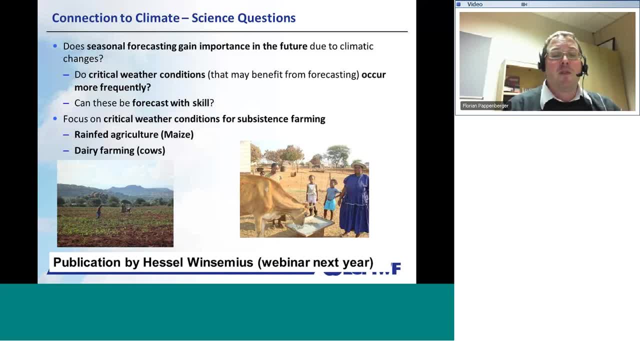 And we've done this with two different critical weather conditions in South Africa for rainfall agriculture, maize and dairy farming. I'm only going to show one quick example here, which is the dairy farming example, In particular the temperature heat index. It basically indicates how stressed 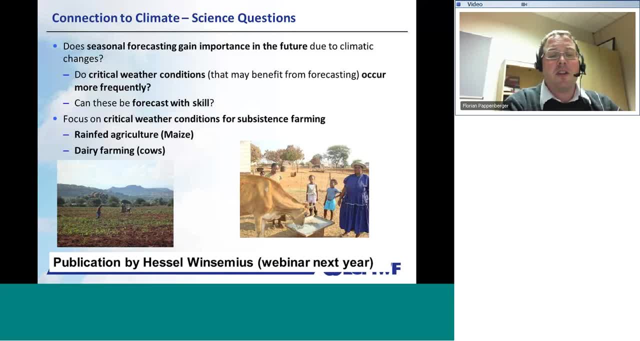 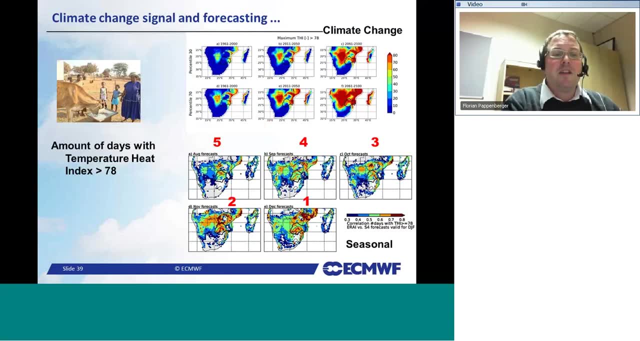 A cow or dairy animal is given a certain heat. The higher the index, the less milk production can be observed. So there's a question that a farmer should build a shed or something to shade a cow On the top. here you see climate change scenarios. 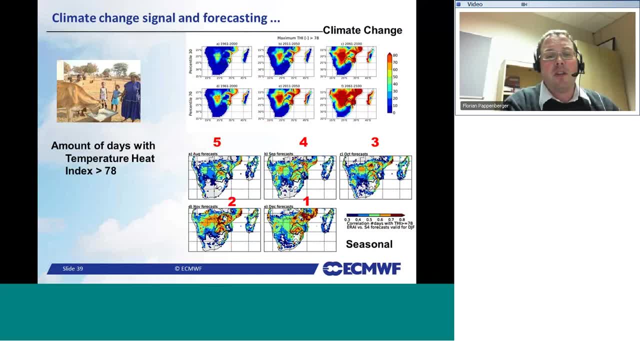 I'm not going to go too much into detail, as I said, Heather's going to talk about it. You could hear a 20 percent and a 70 percentile. We're looking at a heat index above 78. This is the frequency. 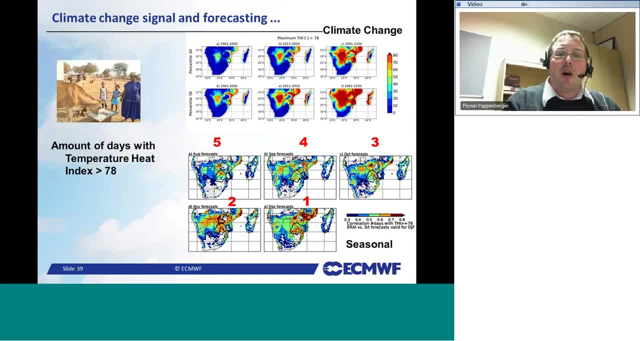 Frequency here or the percentage here, And you can see that from the scenario from 1961 to 2000,. 2011 to 2050, there seems to be an increasing signal. So there seems to be some indication that regional climate models may predict some increased frequency in this particular stress index. 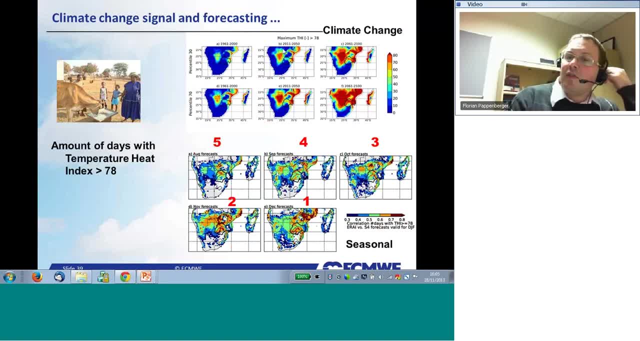 If you now go to, can we actually forecast this index? And here's different forecasts with different lead times: Five days, five months, four months, three months, two months and one month. It shows correlation. The higher the correlation in this particular interpretation, we are more skillful. 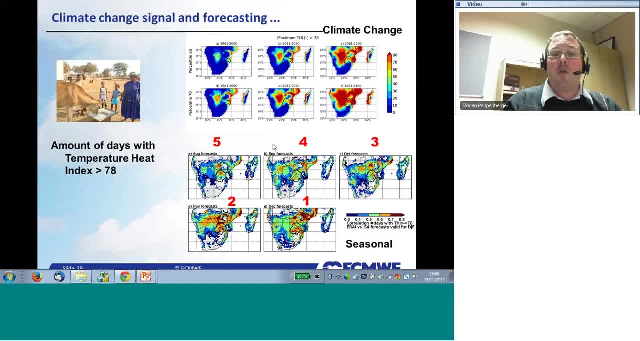 And you can quite nicely see, we are actually also skillful in doing this forecast. So, for this particular example, we can argue that yes, we see a climate change signal And, yes, we are having some skill with this particular skill method to predict. Oops, 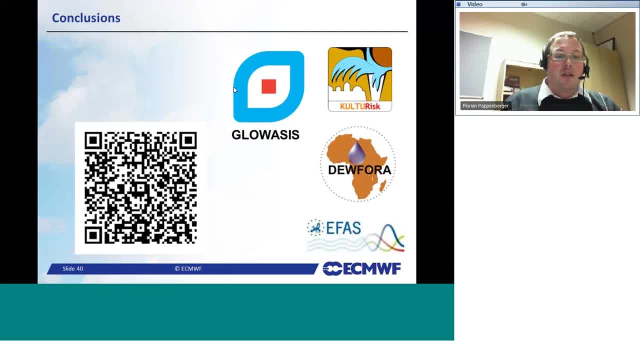 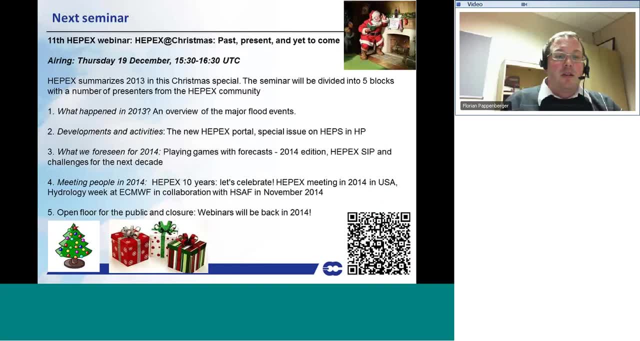 So you can see that this is a very good example of what HAPEX has done in the last years. It will look into the future. It will also give you some more information about meetings we have in the future. It also invites contributions from you. 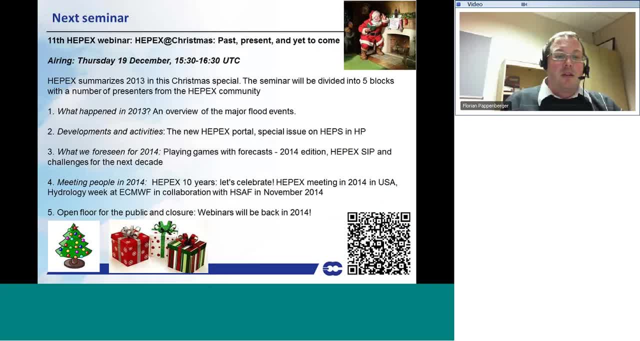 And that's all I wanted to say. Thank you very much, Is that right? Yes, Thank you very much, Florian. I don't know what happened at the end here, because I lost you in my computer. Maybe it was just my problem. 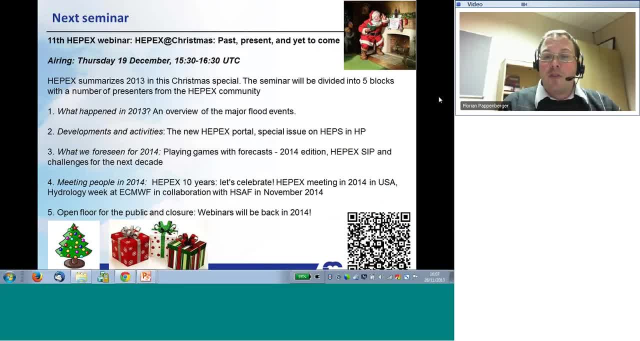 But can you just repeat a little bit on the last slide and the conclusions, And after that I will leave the word free to everybody who wants to have a question. So either you unmute yourself or you send me a chat message. With last slide you mean the HAPEX slide. 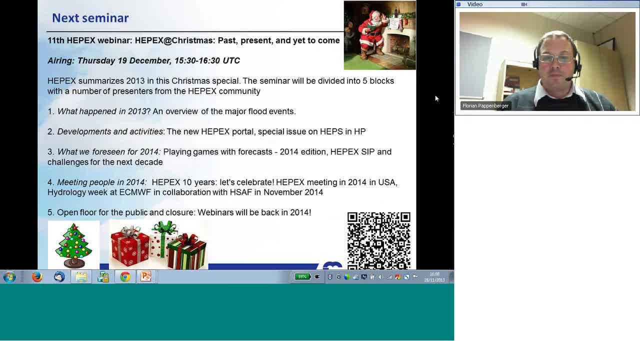 Yes, Okay, Quickly. HAPEX, Christmas, 19th of December 1530.. Drink some mulled wine, Get your Christmas hat and listen to what we are going to do. So we are going to review the past of HAPEX. 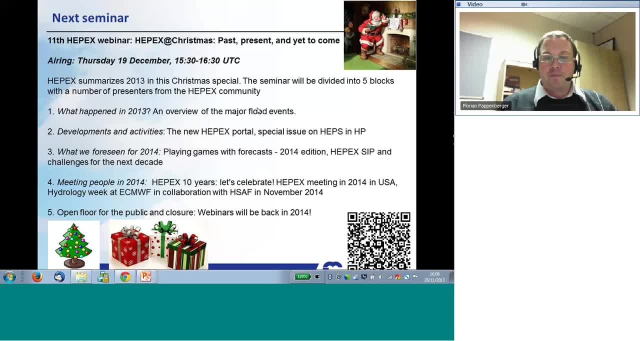 We are going to review the future of HAPEX And we are going to invite you to suggest new things for HAPEX And we are going to tell you what happens next year in terms of meetings. Felix, Okay, Thank you very much. 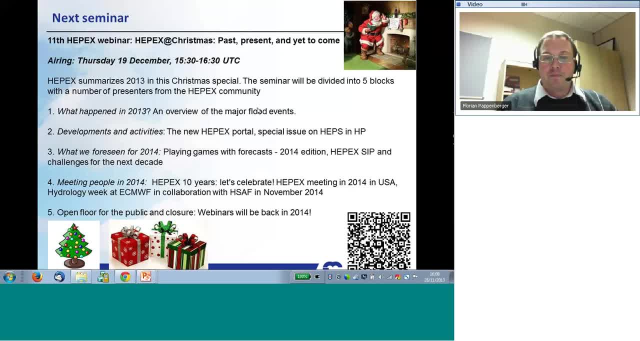 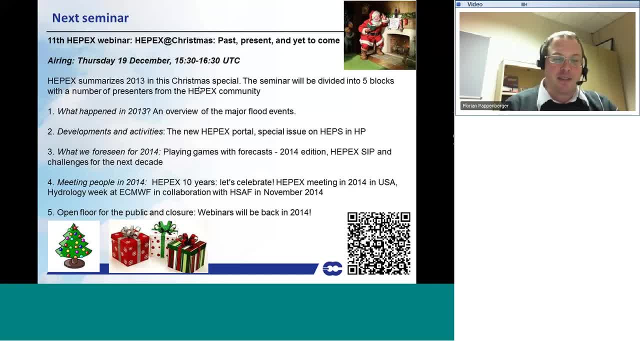 It up to you. There are two questions. It was stated that seasonal forecasting is at least as good as climatology. Would you say this is true? Can you show a map where seasonal is good? Sorry, I can get Great. Thank you. 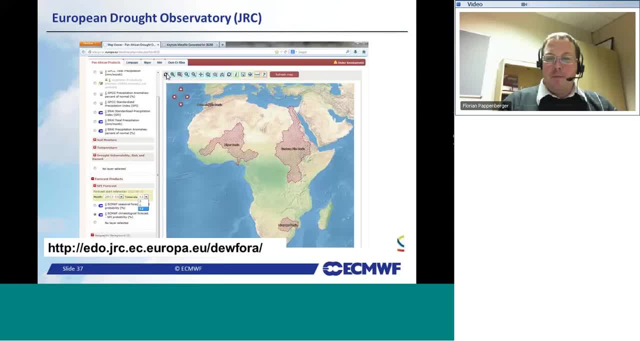 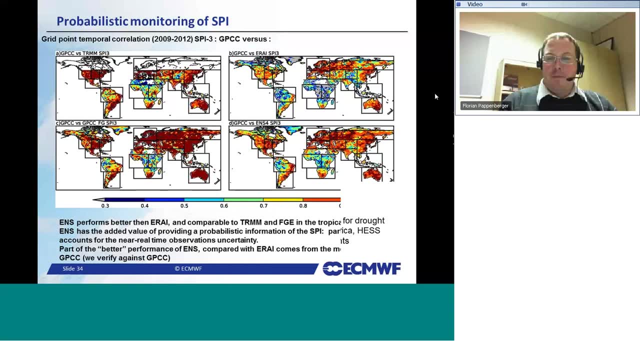 terms of for the African continent in terms of charge forecasting. I haven't got the map here now and in this particular example we could show that seasonal forecast is always at least comparable to climatology. it doesn't always beat climatology. I'm sorry, I haven't. 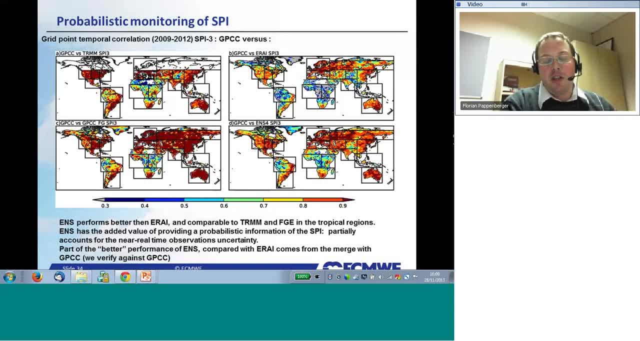 got the map here and we won't need to send you the paper to show you that in more detail. okay, and do you have any more questions from anybody else in the audience? hear me, John. can you repeat that? yes, can you hear me now? we can hear you. yes, okay, uh, I have a question. 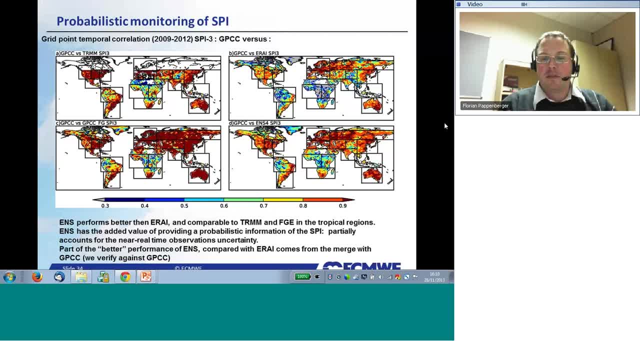 about the seasonal, the monthly and seasonal predictions. I've looked at the monthly and seasonal predictions of precipitation and temperature. that for the United States, NCEP's climate forecast system, their CFS system, the original version of it, version one, and then there's a new version two out. and one thing that I found was 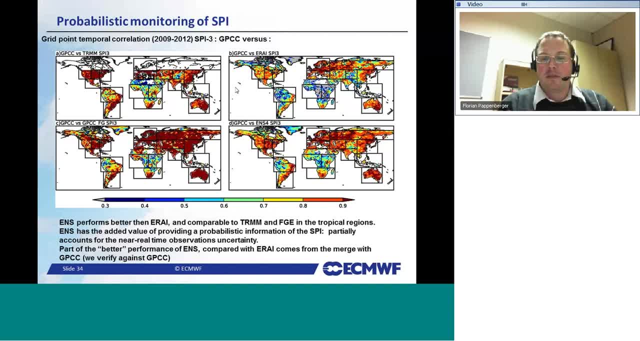 that the correlation between the values that are predicted and observed depend almost completely on the event at when it occurs that you're trying to predict, not the lead time to that event, and there's a very strong seasonal variability in that correlation. so there are times of the year in different locations and these very different. 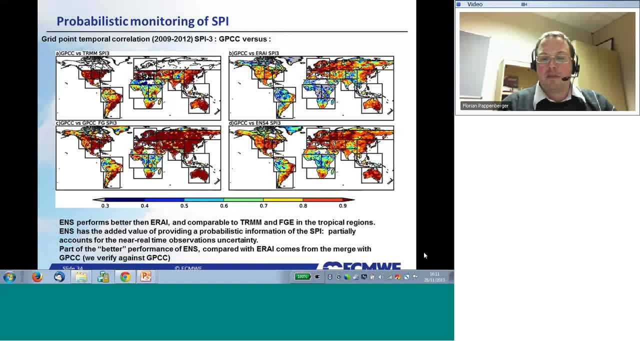 a number of events are happening from place to place. have you seen something like that happen with the ECMWF forecast? I think yes, I haven't. I think seasonal forecasting and monthly forecasting is still a difficult area and skill varies widely and I think one has to be extremely careful because the skill which is, I think, 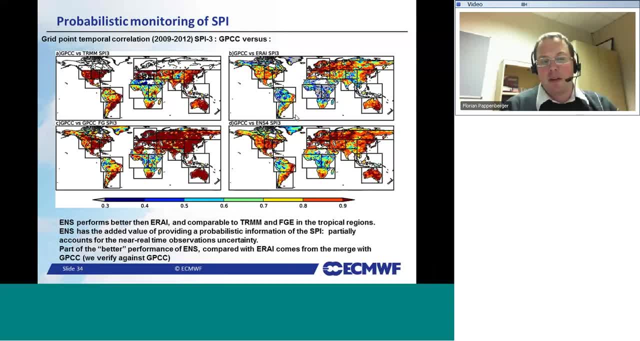 John, you've done the right thing in looking at it yourself, because the skill which is very often represented in the standard skill analysis of those type doesn't necessarily always reflect your application or the way you're going to use it, Particularly hydrology, which may accumulate over space and time quite a bit depending. 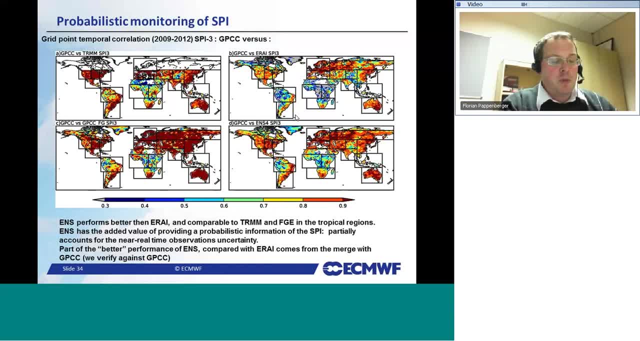 on the catchment. there may be actually some skills sometimes available to you from the seasonal forecast which is not necessarily as apparent if you look in a grid box by grid box accumulation Right. By the way, I also found that the seasonal three-month predictions were a lot more skillful. 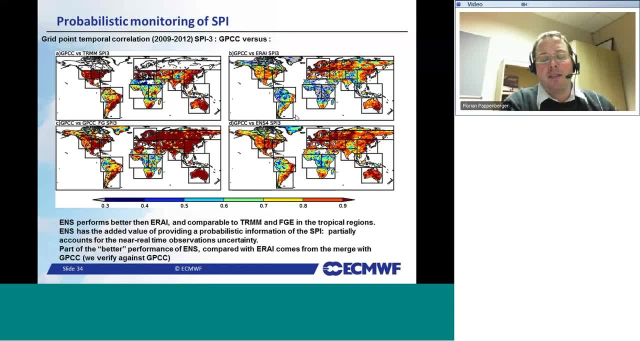 than the monthly ones. The monthly ones can be very noisy, but the seasonal, the three months, tends to definitely show a better skill. I think our experience is a bit different. Our experience is that the prediction of the monthly forecast tends to outperform the 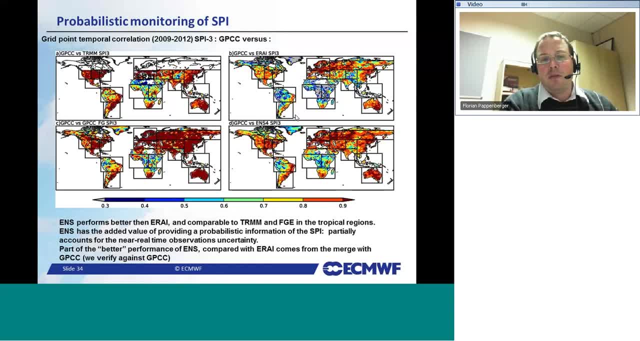 seasonal forecast, and there are several reasons for that. I think the most important one is that probably the monthly forecast gets updated twice a year in terms of model and data simulation and so forth, whereas the seasonal forecast tends to be a more frozen system. So you've got certain incarnations, because one, two, three and four, so it can't be a 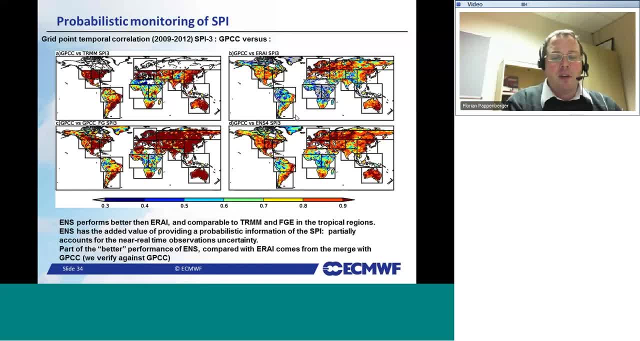 seasonal system Four is similar to CFS system one and two. So if you're actually going the opposite way, we actually believe it would be beneficial in merging the monthly forecast with the seasonal forecast, and Francesca Di Giuseppe has recently published a paper where she shows how you could do that, and we believe that actually. 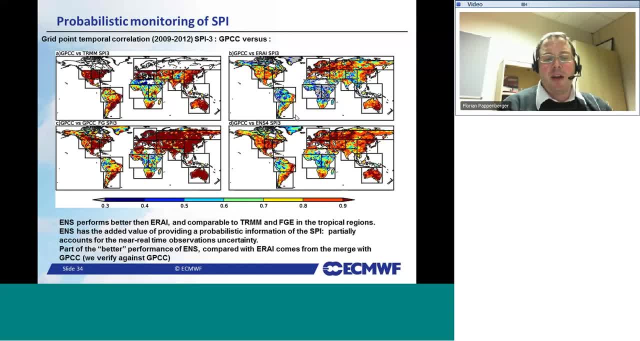 we can increase skill by using the monthly forecast as well as the seasonal forecast together. Of course, it's quite a difficult task to merge the two, because they all have different ensemble members which have to be joined up. They have to be somehow selected. They have to be somehow selected. 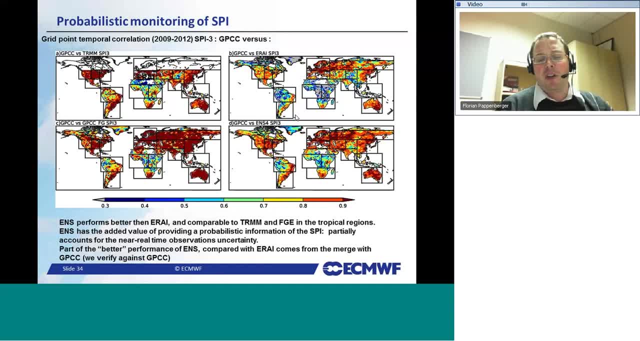 It's like a different statistically. so it's actually not that simple, I think. But I do believe that the monthly forecast- at least the results I've seen so far- are of higher skill than the first month of the seasonal forecast. Seasonal forecast, also at ECWF, is at a causal scale than the monthly forecast, so it also 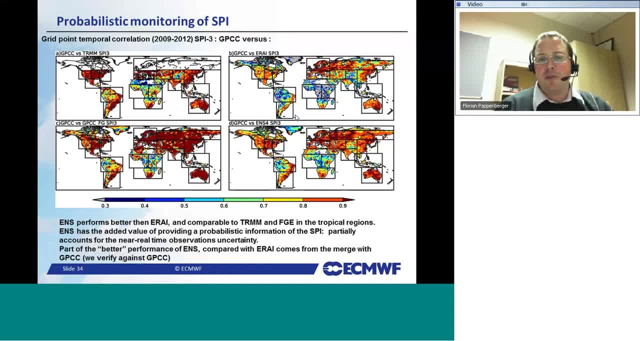 contributes. There's many other factors which contribute, which I probably don't all know myself. to say, Yeah, that sounds very interesting. I think it would be nice to find out. It would be nice to find out why this happens, why you're getting the results you did. 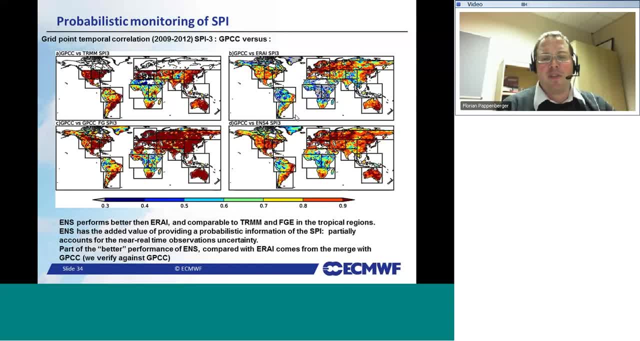 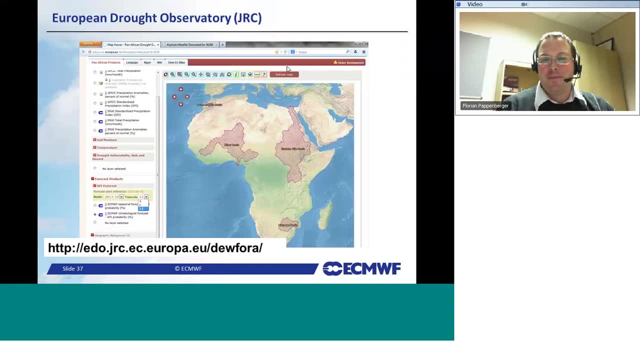 What I talked about. all the forecasts came out of an ensemble prediction or just a single value prediction, where we use several dates in the past- single values- to create the ensemble, But the ensembles used were exactly the same for monthly and seasonal prediction. 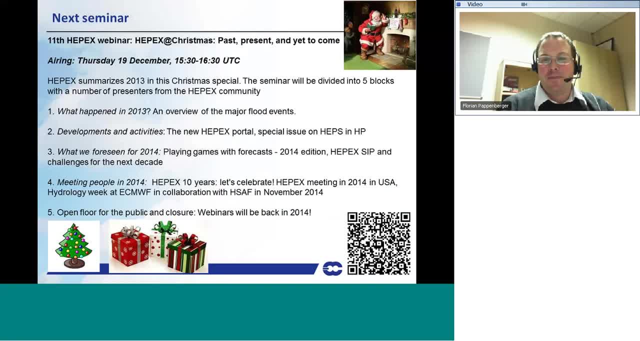 We didn't have a separate model. Yeah, Yeah, We didn't try to use any empirical indices or anything else to improve this, So there's a lot of things to be looked at here, and trying to understand why you're getting the results you're getting would be interesting, I think, too. 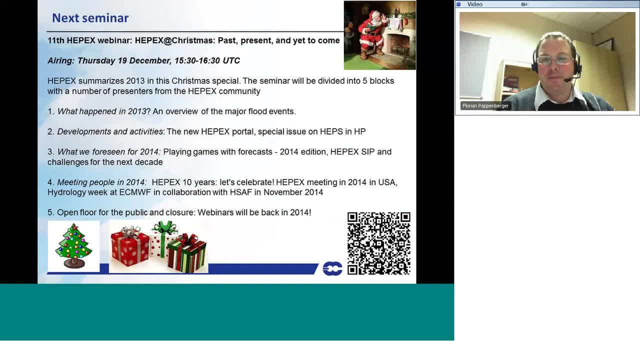 I fully agree. Okay, thank you, John and thank you Florian. We also have another question, another question from Mike, Going back again to the climatology. So could you back up a little bit? Yeah, Yeah, Can you explain a bit more on where it could be, modes where the seasonal forecast is worse. 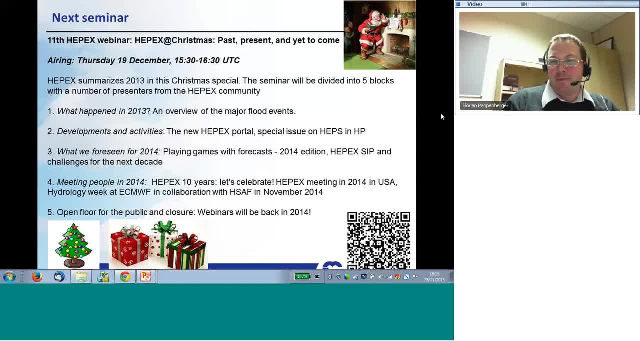 than climatology. We believe this could be the case, particularly when the seasonal forecast drifts and you don't correct for that one, And maybe Mike is right, or make a two-seating statement, But I do think it belongs on the. it really depends on the variable as well as the region. 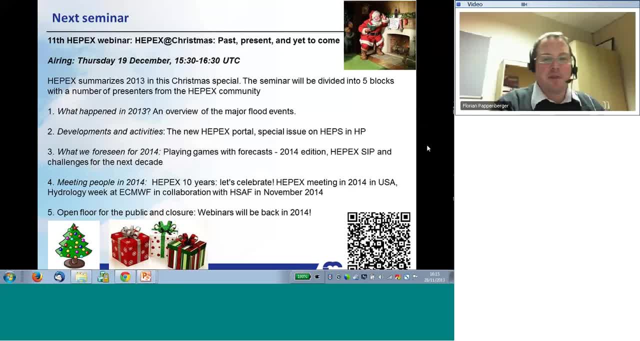 Okay, So for our particular case, in terms of drought application, that this was not the case. But Mike is absolutely right that one needs to look and very often this is not necessarily the general case and it may well be sometimes different. Okay, do we have any more questions?